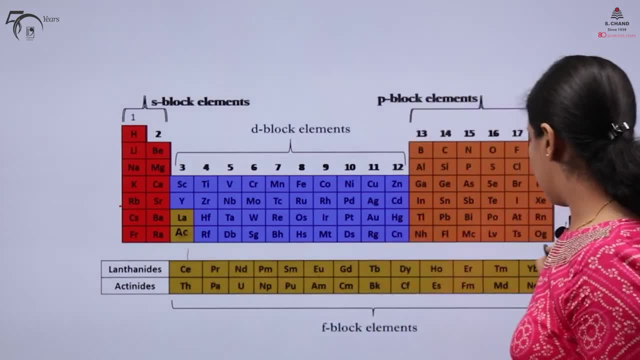 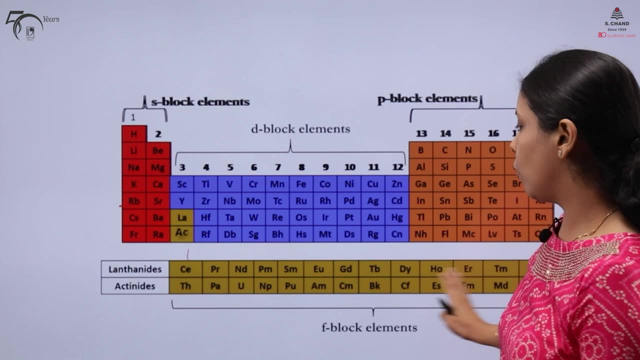 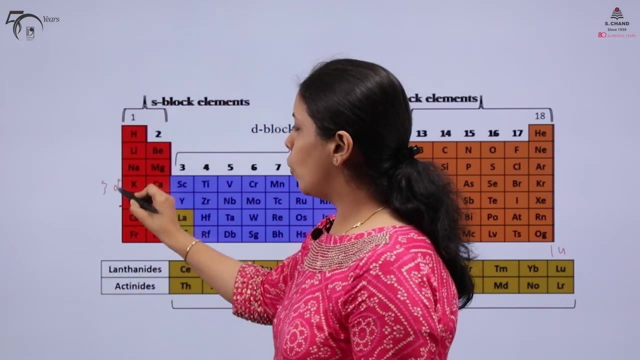 These are getting filled from 1 till 14.. It is getting filled over here, So these are known as lanthanides, and the actinides are getting filled from thorium to laurentium, So this is getting filled after actinium. So this is our 3D, 4D, 5D and 6D, So 6D element. 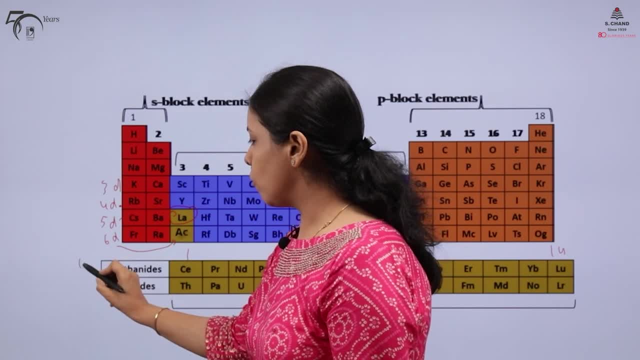 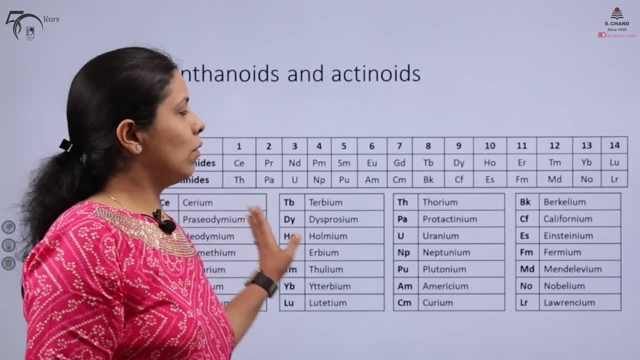 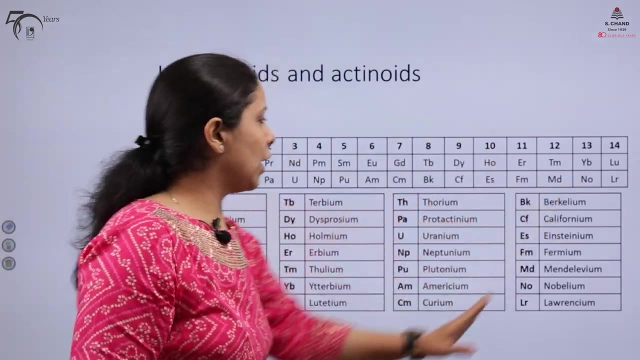 and 5D element. So after 5D it is getting 4F, electrons are getting filled and after 6D, 5F elements are getting filled. So if you see over here, these are lanthanides, actinides. as I have told you, 14 elements are getting filled, from cerium to lutetium. So this is. 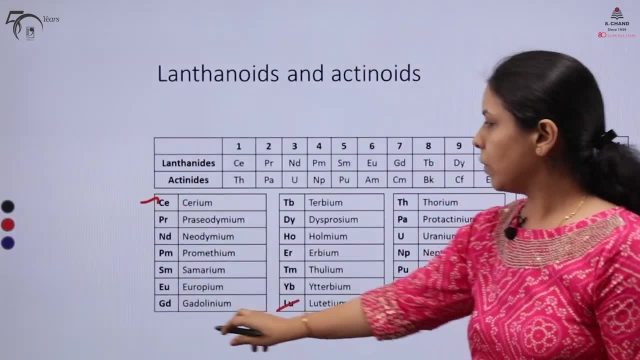 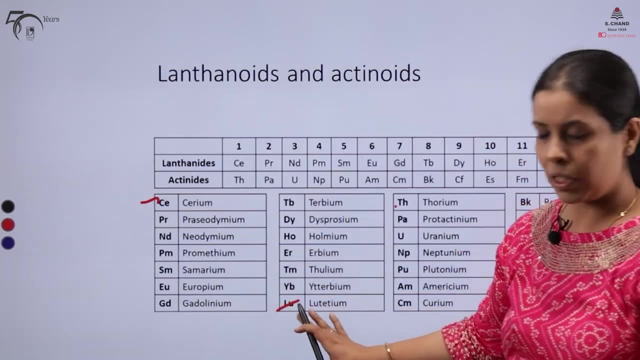 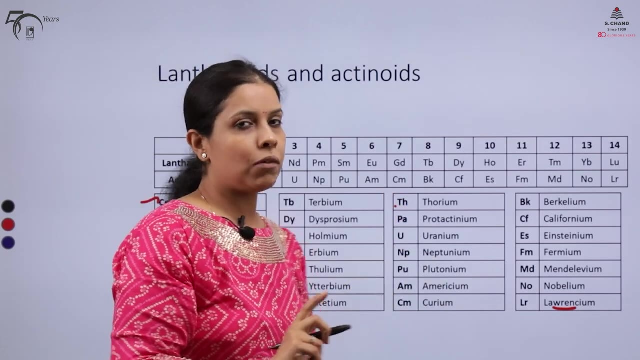 our cerium. this is cerium till lutetium. these are our lanthanides, and from thorium to laurentium is our actinides. So these 14 elements- I have written the name for your convenience- These are our lanthanides. From thorium to laurentium are our actinides, And I told you in the previous. 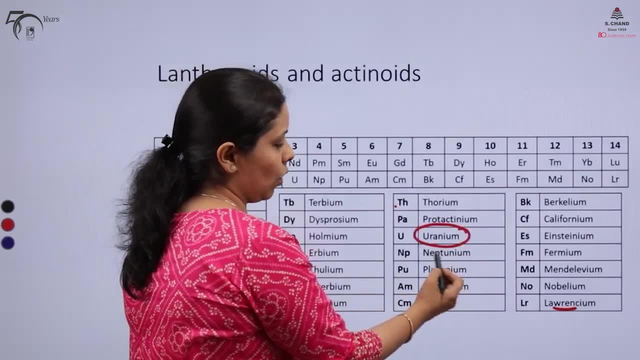 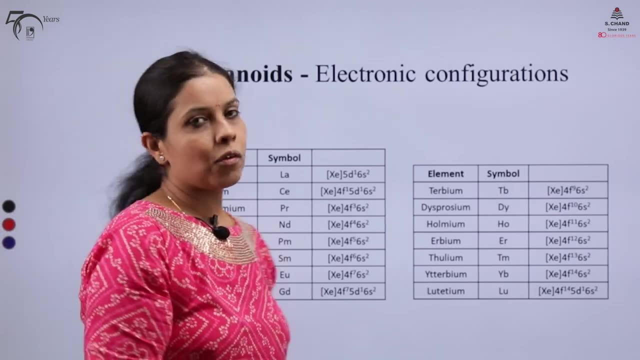 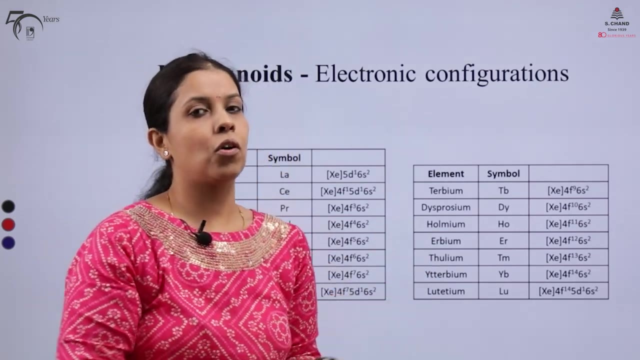 starting of the video that after uranium, all these elements mostly are man-made. They are not naturally occurring elements. So we will start with the properties of lanthanides. and the most important thing to understand before we go into the properties is electronic configuration. that is how electrons are getting adjusted in these orbitals. So how do they get adjusted? 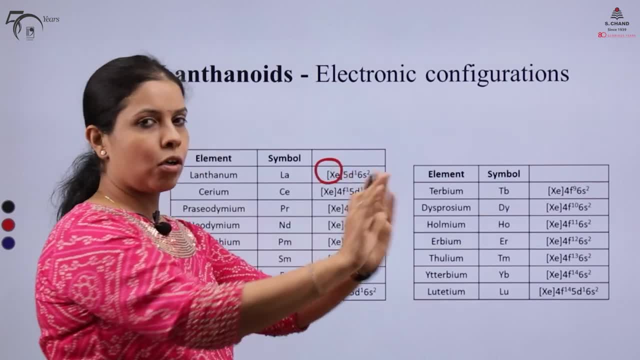 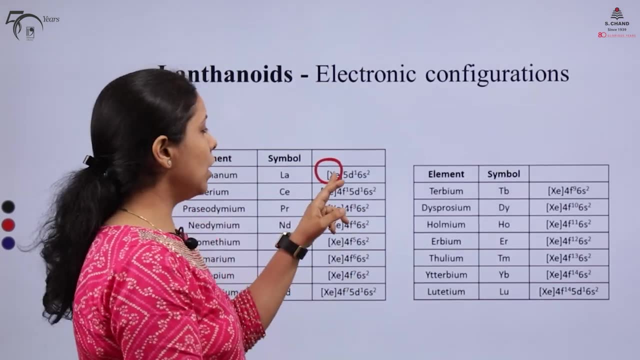 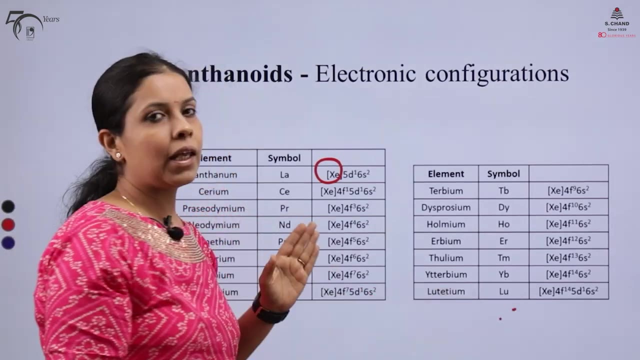 The first lanthanum is xenon. your noble gas configuration has been attained. After that, 6-2 electrons came and the first 5-D one came. So what happened to its electronic configuration? 5-D1, 6-X2.. After that, we know when lanthanides will start then, from cerium to lutetium, our 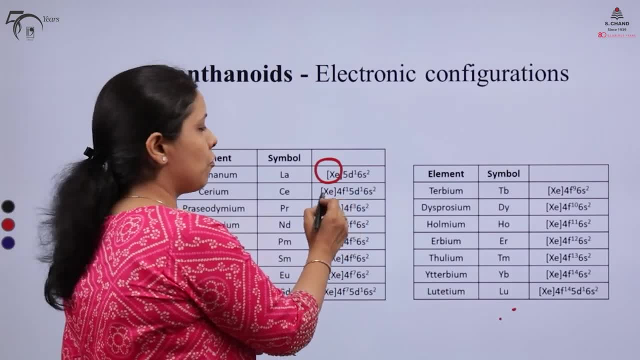 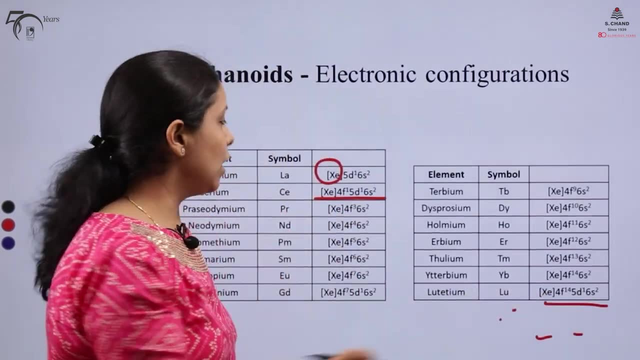 4-F electrons will be filled. So what will happen? 4-F1,, 5-D1, 6-X2 and what will happen to lutetium 4-F14,, 5-D1 and 6-X2.. So that means our 4-F electrons have started to be filled, but the 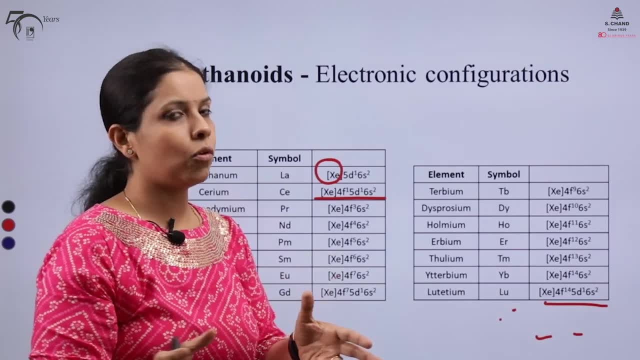 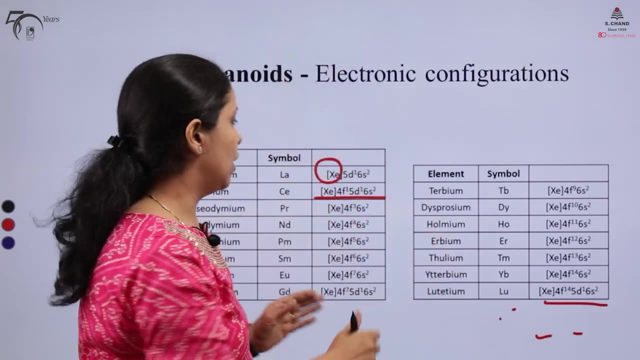 energy of 4-F and 5-D More or less same. So sometimes what happens is electrons go to 4-F instead of 5-D, which stabilizes the energy for it. So 5-D will come to 4-F sometimes. So you will see the. 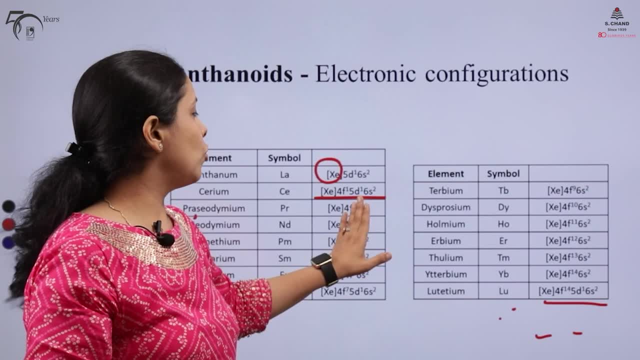 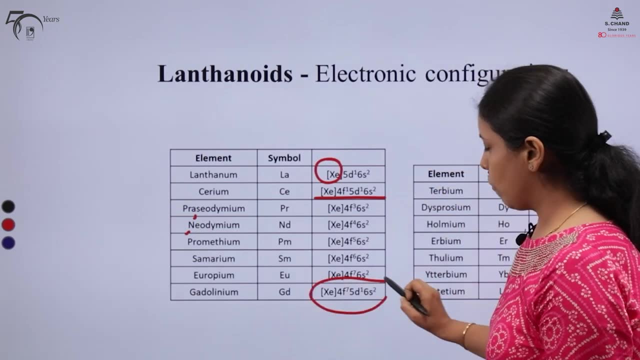 next element of cerium. its configuration will not be 4-F2, 5-D1, but it will be 4-F3.. Now the next thing to see is: why is it of gadolinium? 4-F7,, 5-D1,, 6-X2.. So you will. 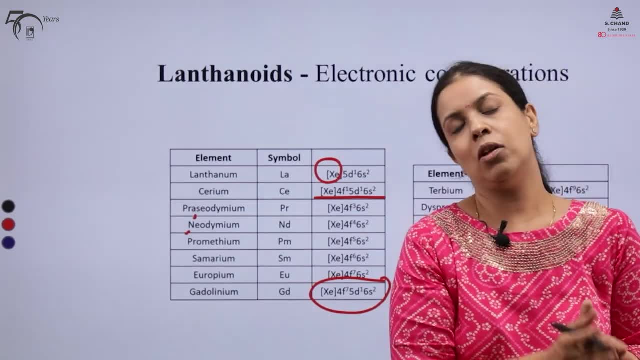 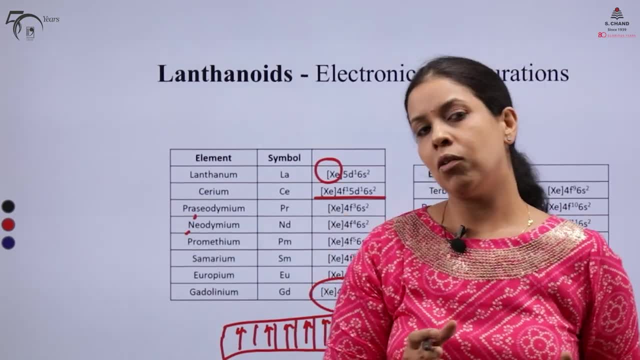 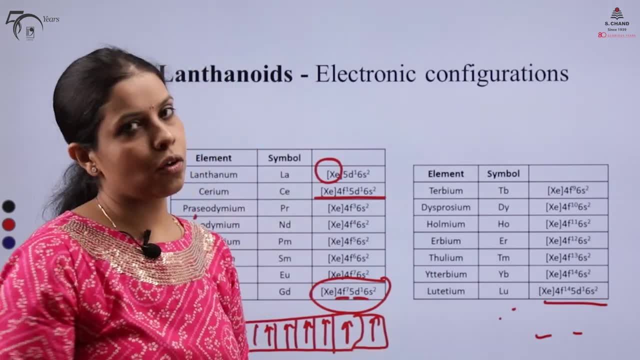 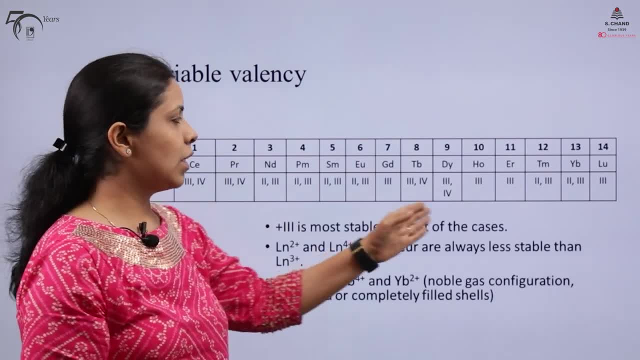 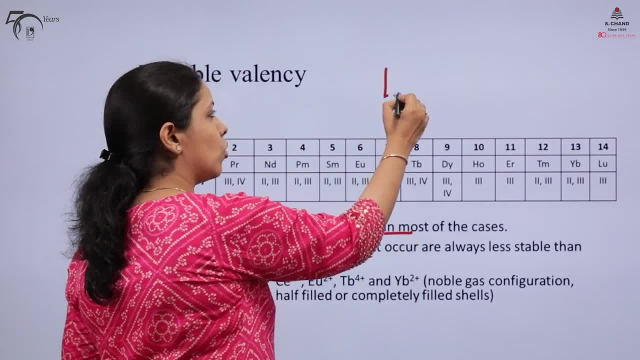 half filled or which is completely filled. So you will remember that we had done it during the transition element series: that half filled or which is completely filled. So you will remember that we had done it during the transition element series- that half filled or which is completely filled. So you will remember that we had done it during the transition. 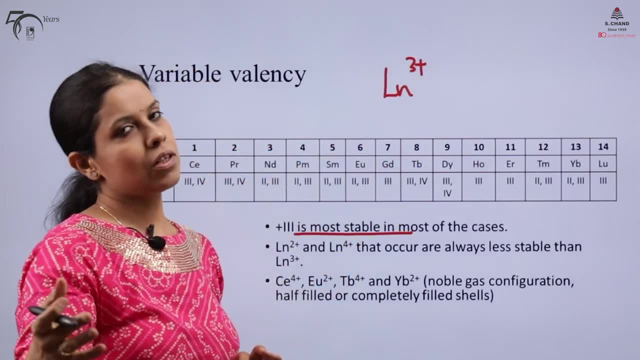 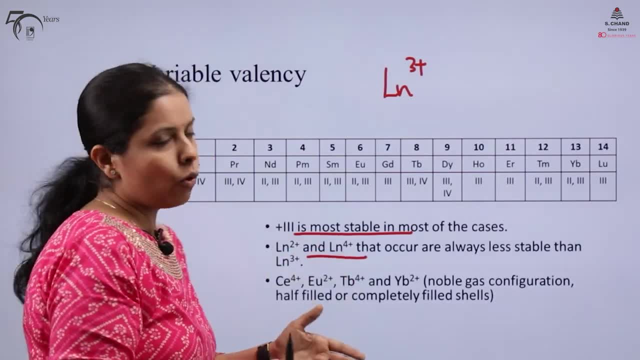 half filled or which is completely filled. So you will remember that we had done it during the transition element series: that half filled or which is completely filled. So you will remember that we had done it during the transition element series- that half filled or which is completely filled. So you will remember that we had done it during the transition. 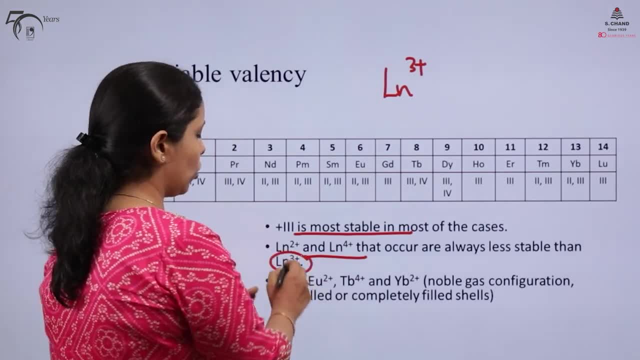 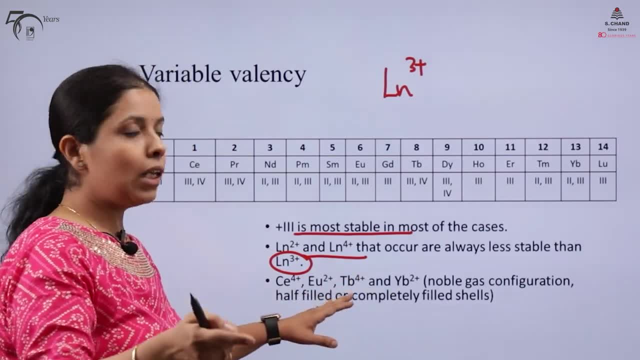 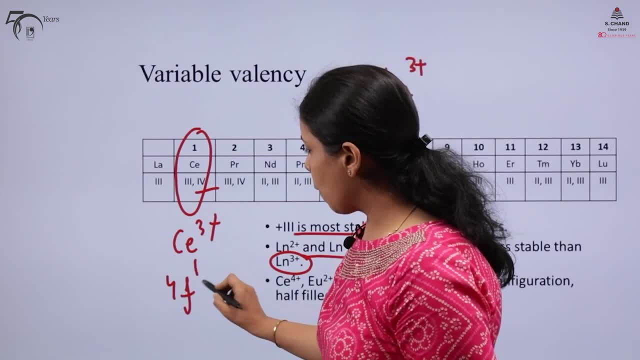 half filled or which is completely filled. So you will remember that we had done it during the transition element series: that half filled or which is completely filled. So you will remember that we had done it during the transition element series- that half filled or which is completely filled. So you will remember that we had done it during the transition. 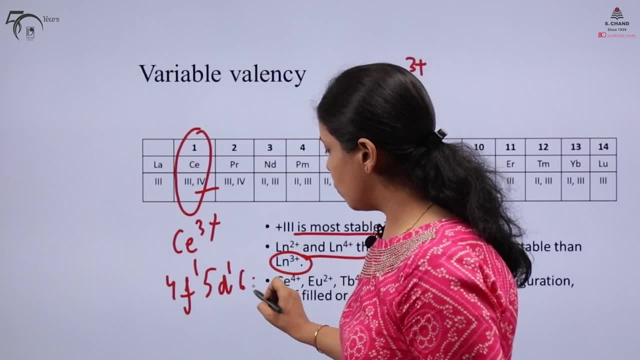 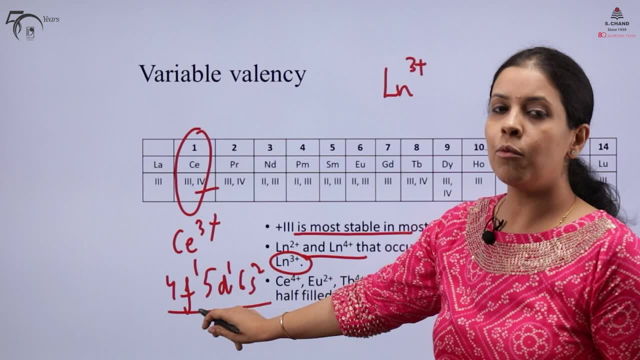 half filled or which is completely filled. So you will remember that we had done it during the transition element series: that half filled or which is completely filled. So you will remember that we had done it during the transition element series- that half filled or which is completely filled. So you will remember that we had done it during the transition. 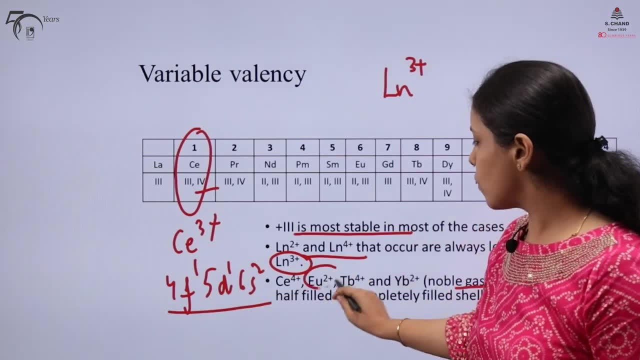 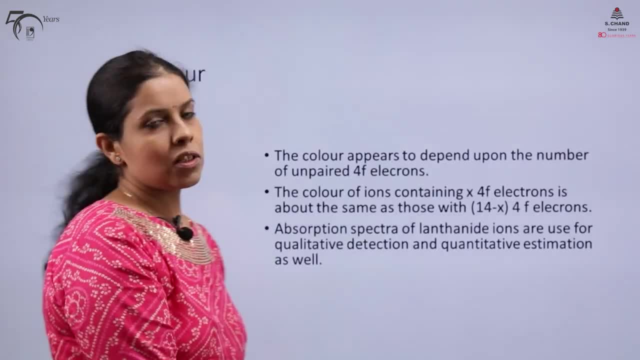 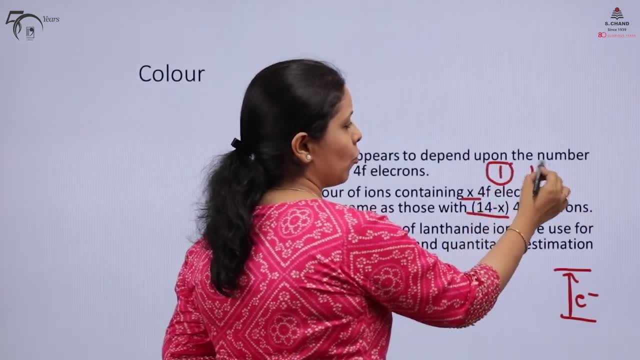 half filled or which is completely filled. So you will remember that we had done it during the transition element series: that half filled or which is completely filled. So you will remember that we had done it during the transition element series- that half filled or which is completely filled. So you will remember that we had done it during the transition. 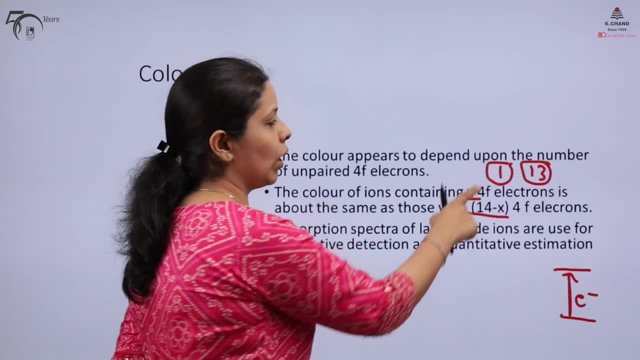 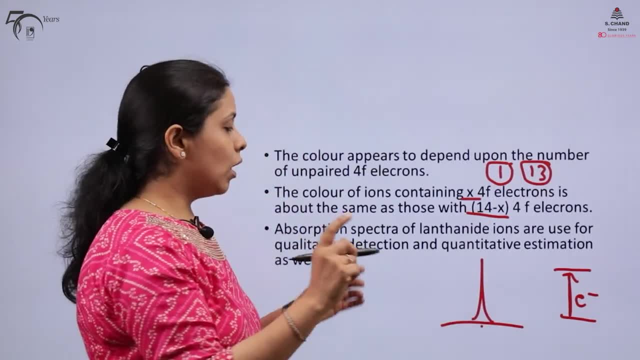 half filled or which is completely filled. So you will remember that we had done it during the transition element series: that half filled or which is completely filled. So you will remember that we had done it during the transition element series- that half filled or which is completely filled. So you will remember that we had done it during the transition. 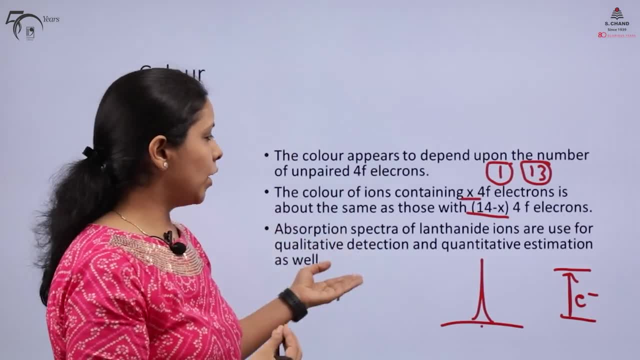 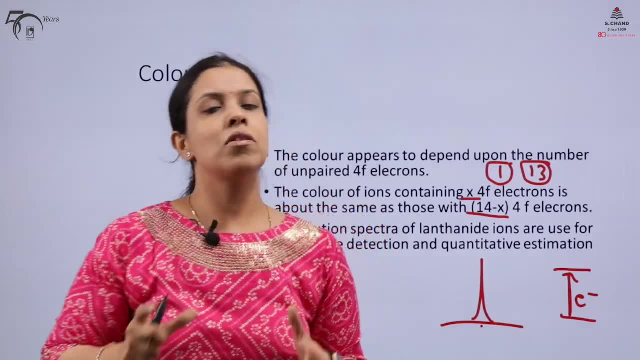 half filled or which is completely filled. So you will remember that we had done it during the transition element series: that half filled or which is completely filled. So you will remember that we had done it during the transition element series- that half filled or which is completely filled. So you will remember that we had done it during the transition. 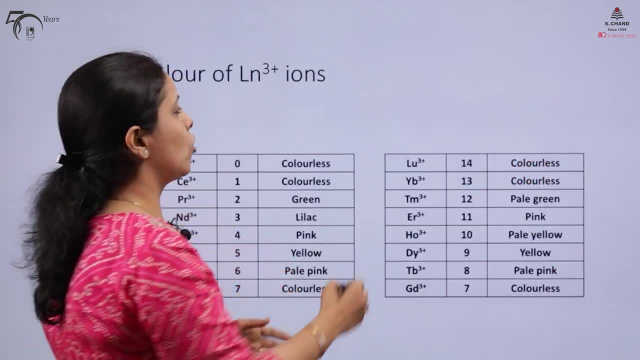 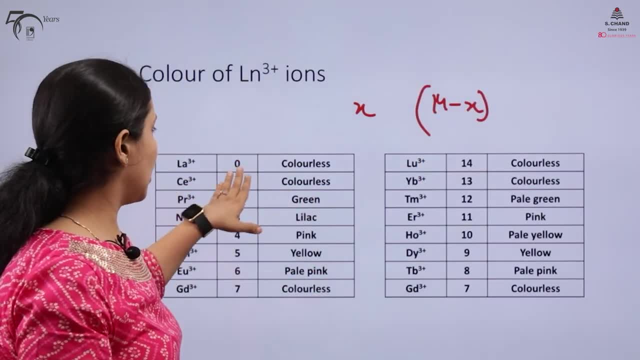 half filled or which is completely filled. So you will remember that we had done it during the transition element series: that half filled or which is completely filled. So you will remember that we had done it during the transition element series- that half filled or which is completely filled. So you will remember that we had done it during the transition. 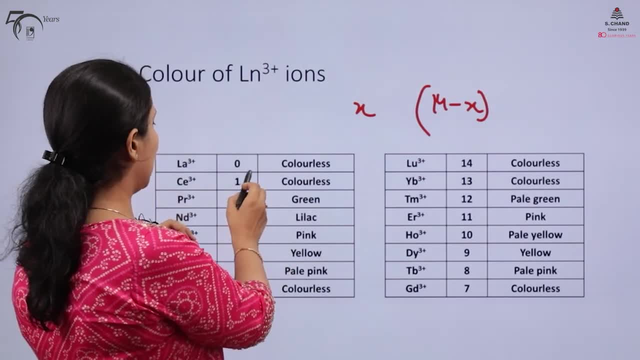 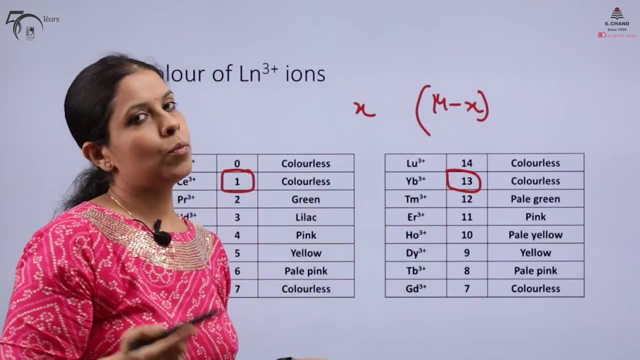 half filled or which is completely filled. So you will remember that we had done it during the transition element series: that half filled or which is completely filled. So you will remember that we had done it during the transition element series- that half filled or which is completely filled. So you will remember that we had done it during the transition. 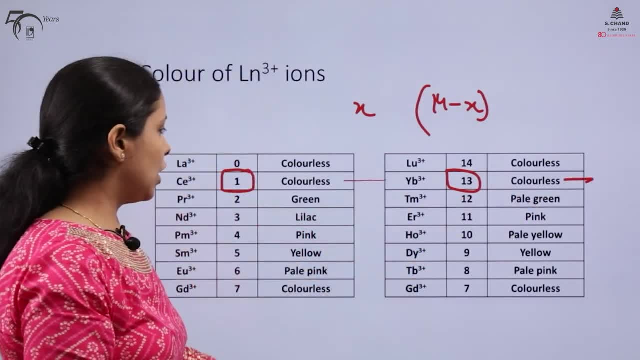 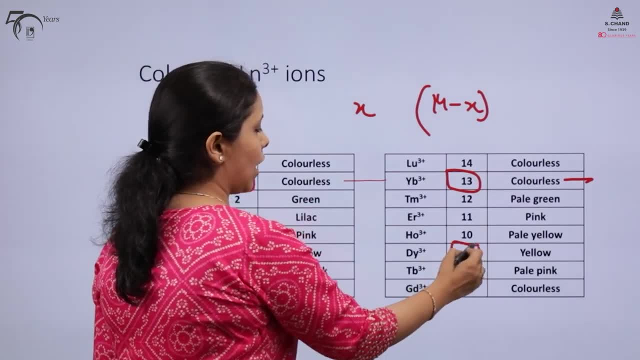 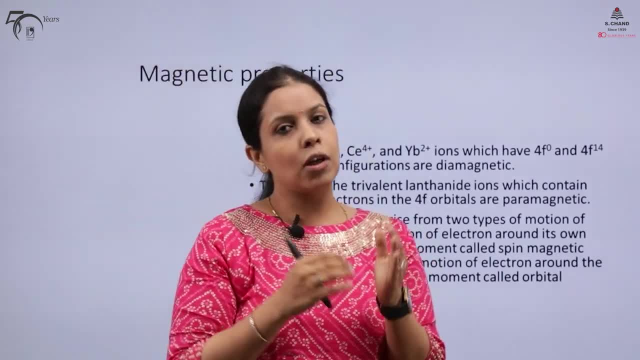 half filled or which is completely filled. So you will remember that we had done it during the transition element series: that half filled or which is completely filled. So you will remember that we had done it during the transition element series- that half filled or which is completely filled. So you will remember that we had done it during the transition. 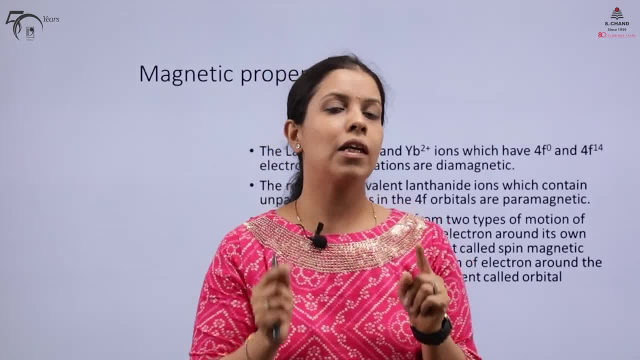 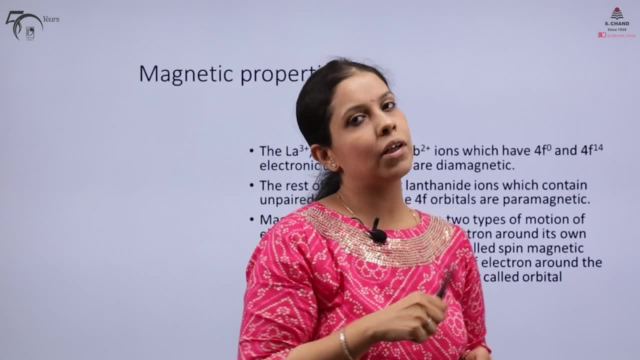 half filled or which is completely filled. So you will remember that we had done it during the transition element series: that half filled or which is completely filled. So you will remember that we had done it during the transition element series- that half filled or which is completely filled. So you will remember that we had done it during the transition. 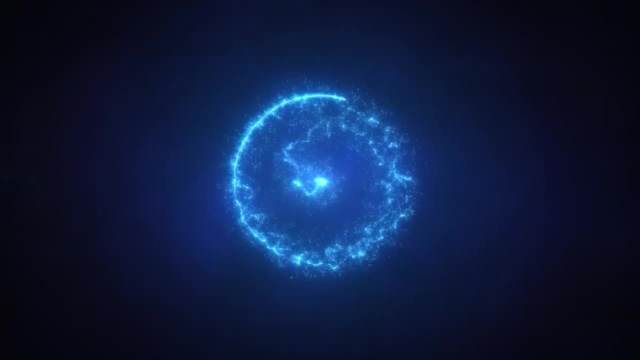 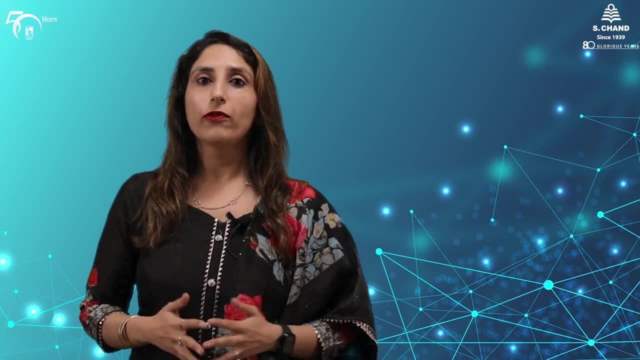 half filled or which is completely filled. So you will remember that we had done it during the transition element series: that half filled or which is completely filled. So you will remember that we had done it during the transition element series- that half filled or which is completely filled. So you will remember that we had done it during the transition. 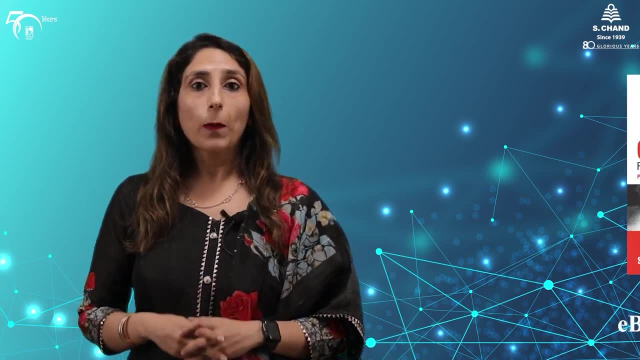 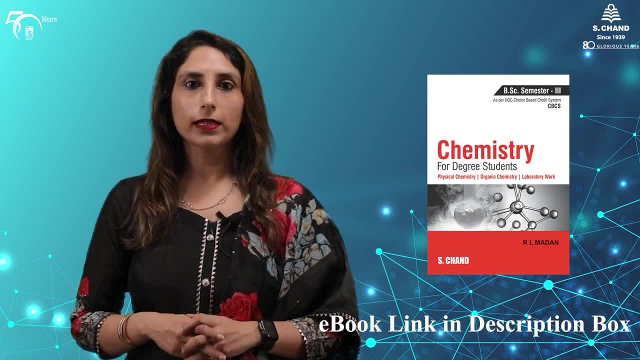 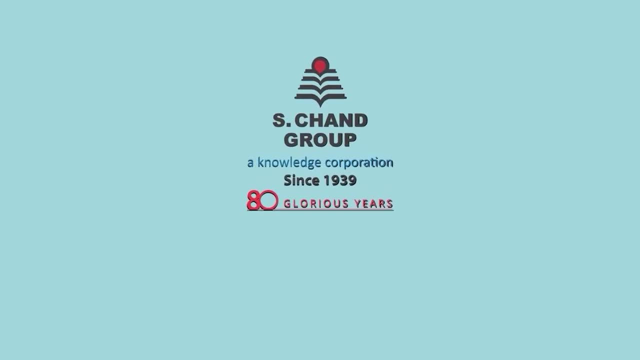 half filled or which is completely filled. So you will remember that we had done it during the transition element series: that half filled or which is completely filled. So you will remember that we had done it during the transition element series- that half filled or which is completely filled. So you will remember that we had done it during the transition. 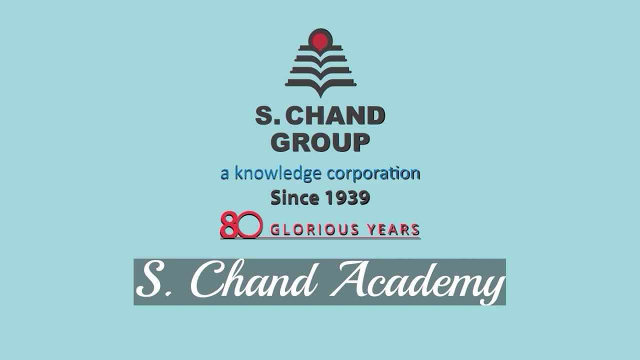 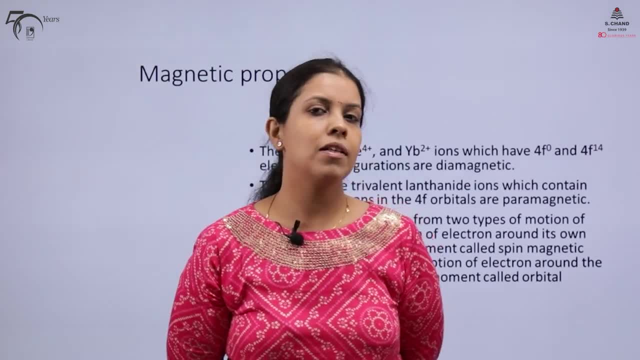 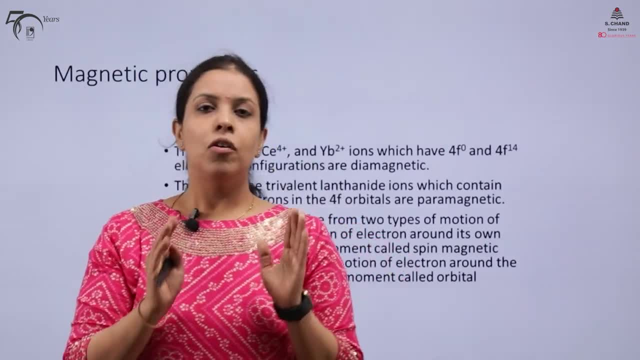 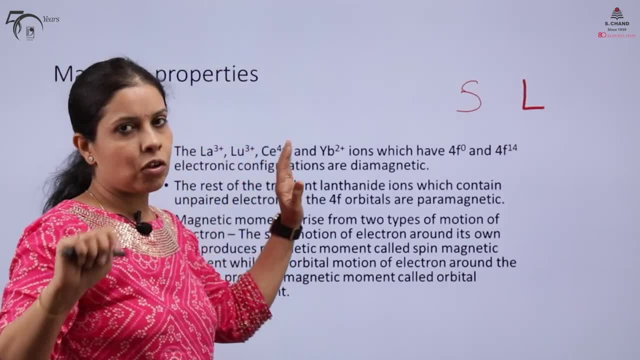 half filled or which is completely filled. So you will remember that we had done it during the transition element series: that half filled or which is completely filled. So you will remember that we had done it during the transition element series- that half filled or which is completely filled. So you will remember that we had done it during the transition. 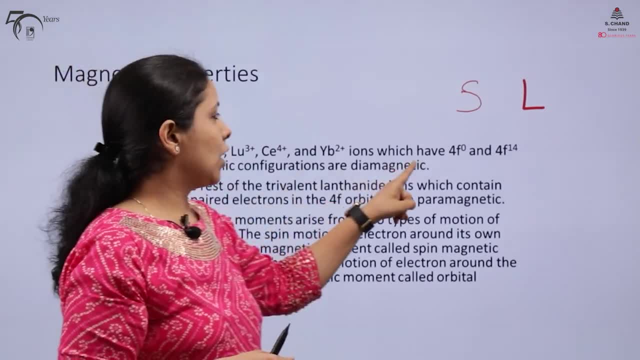 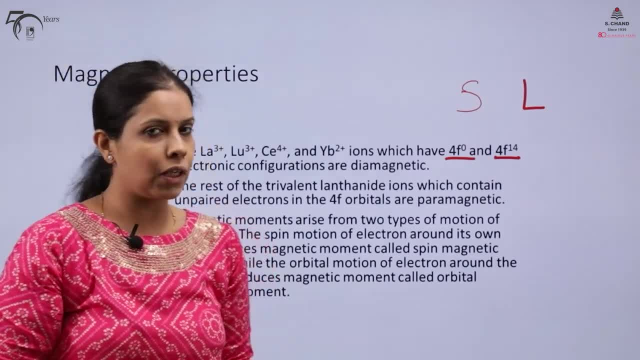 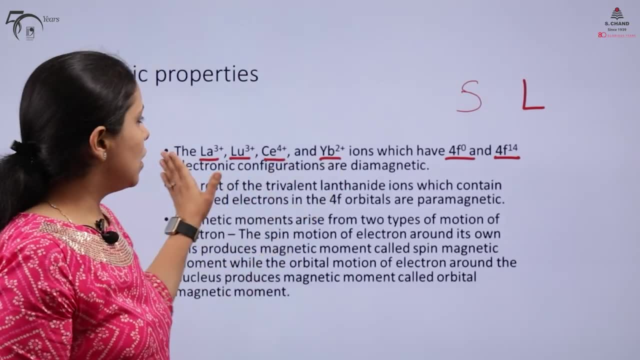 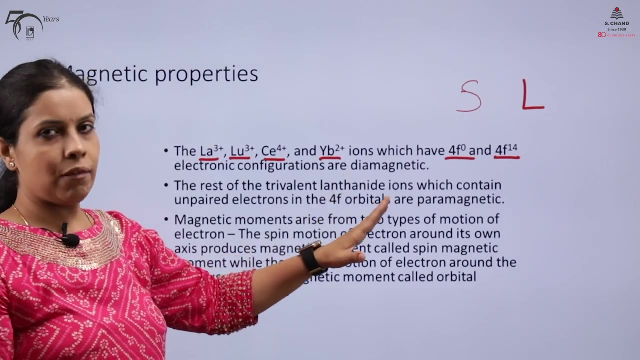 so even in that there are no unpaired electrons due to which the magnetic field will be generated. So all these configurations- LA3+, LU3+, Serium 4+ or Terbium 2+, these are all having configuration 4F0 and 4F14, so they are diamagnetic in nature. So rest of the trivalent lanthanides: 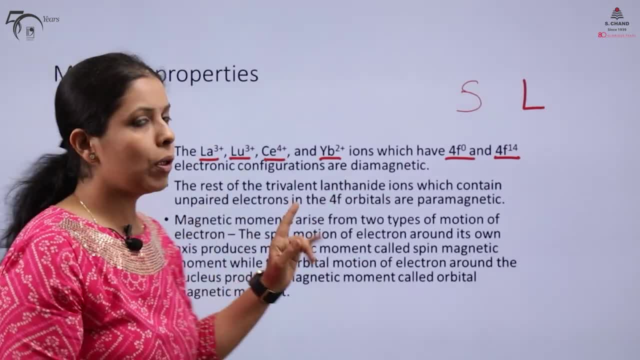 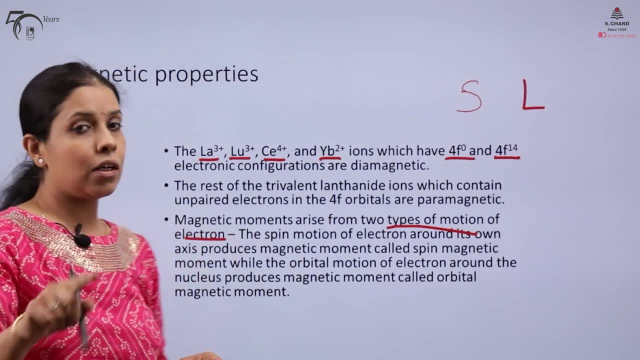 ion, which are having unpaired electron, so they will be paramagnetic in nature. So I ask you this question: what are the two types of motions of electrons which are responsible for giving us the magnetic field? The spin motion of electrons around its own axis. it. 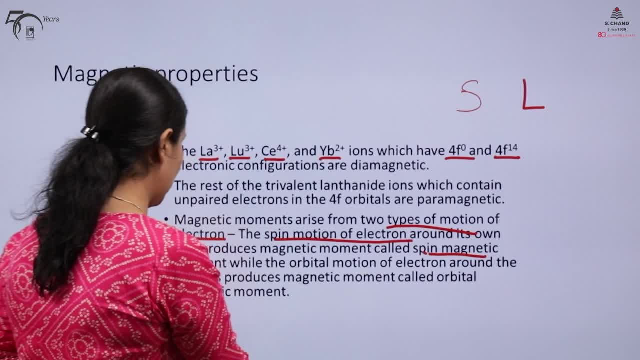 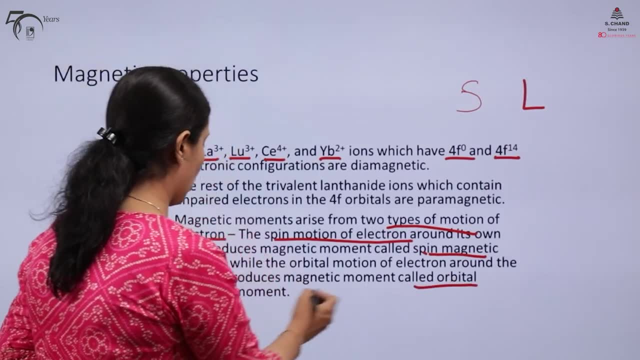 produce magnetic moment, which we call spin magnetic moment, while the orbital motion of electrons around its own axis, it produce magnetic moment, So this is called spin magnetic moment. The movement which is produced around the nucleus produces magnetic field, which is known as orbital magnetic moment. right, So there are two types of motions: spin magnetic. 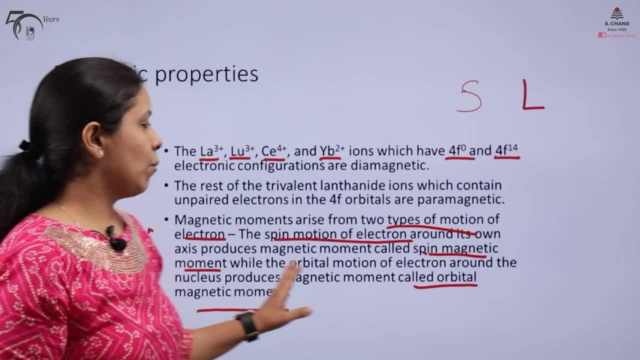 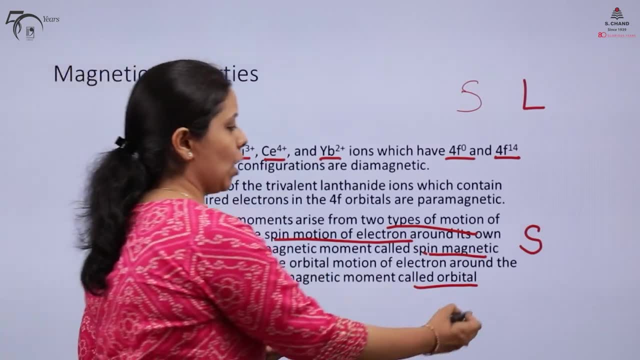 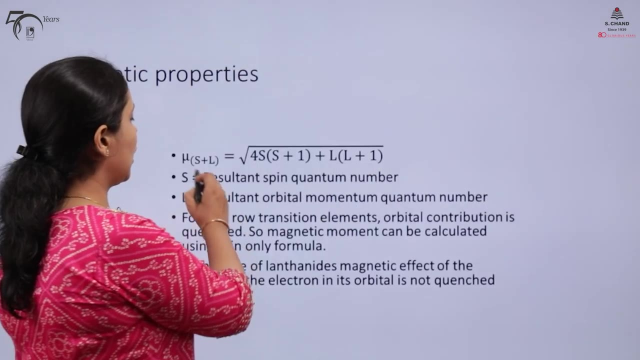 moment and orbital magnetic moment. So spin magnetic moment gives us a quantum number which we call resultant spin quantum number. For orbital magnetic moments, we get an orbital angular quantum number which is known as L, denoted by L. So when we have to get out, 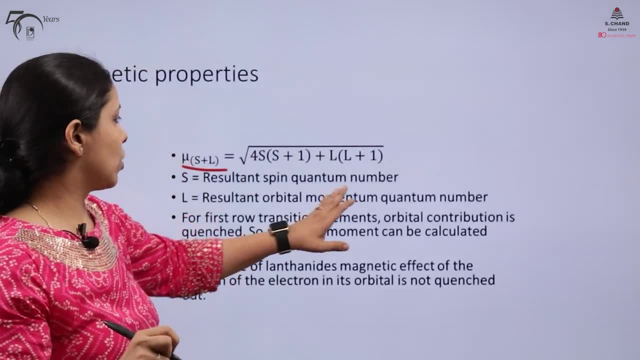 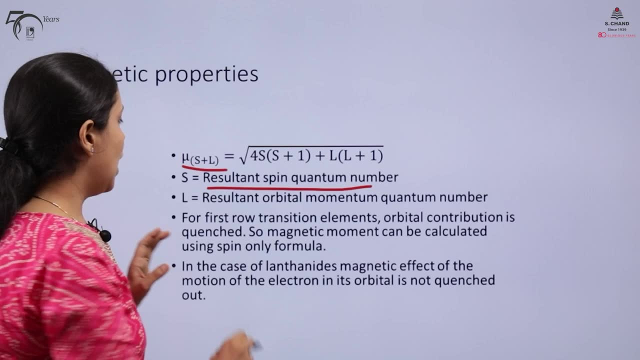 We have to use spin quantum number as well as angular quantum number, So we will use this formula for expanded form. So S is resultant spin quantum number, L is resultant orbital momentum quantum number. So by using these two we can get the magnetic moment. 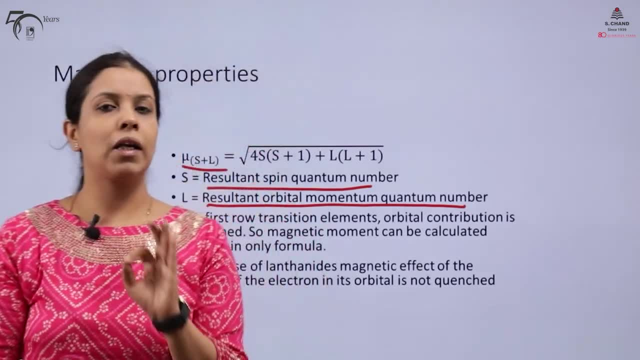 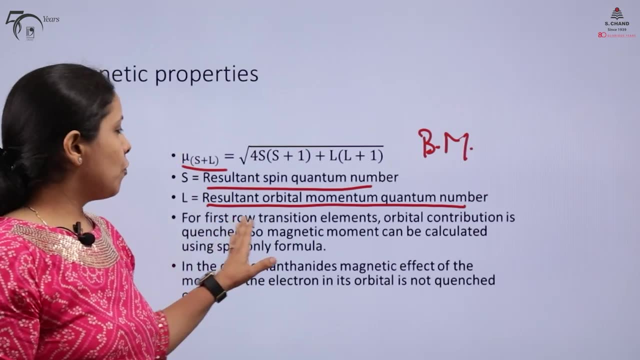 If you remember the unit of magnetic moment, then we will get it in the form of Bohr magneton, which is represented as BM. Right, Okay, So for the first row transition element. now I am not talking about the lanthanide series. 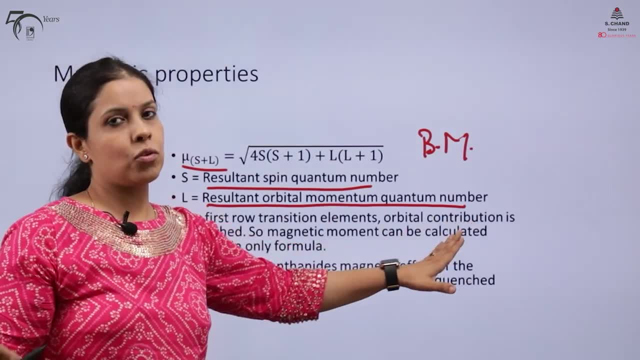 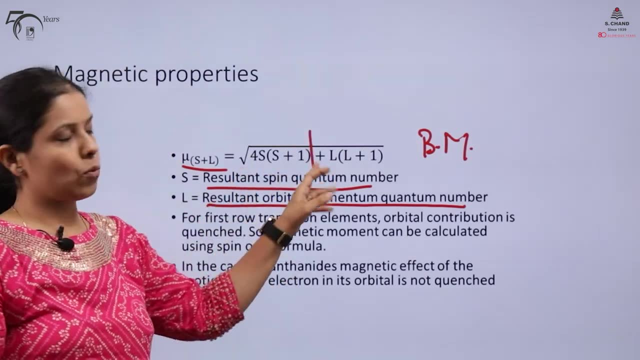 In the case of transition elements, the orbital contribution is quenched, So we can remove it. We can remove it, So we only use this formula till here: 4S S plus 1.. But this does not happen in the lanthanide series. 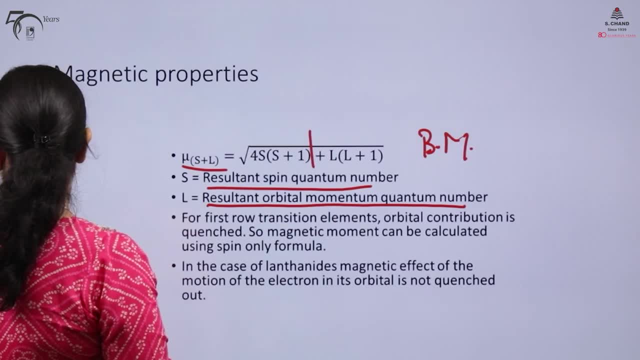 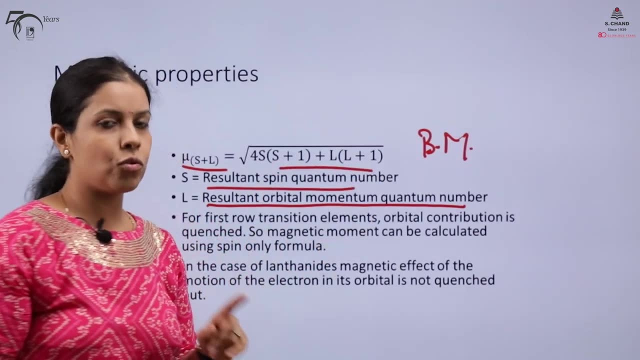 We have to include orbital contribution. So to include orbital contribution, we have to use this proper formula, which we can use by writing this formula: In the case of lanthanides magnetic field, the effect of motion of electron in its orbital is not quenched. 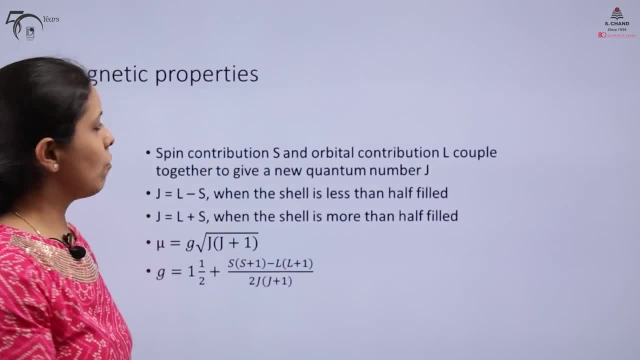 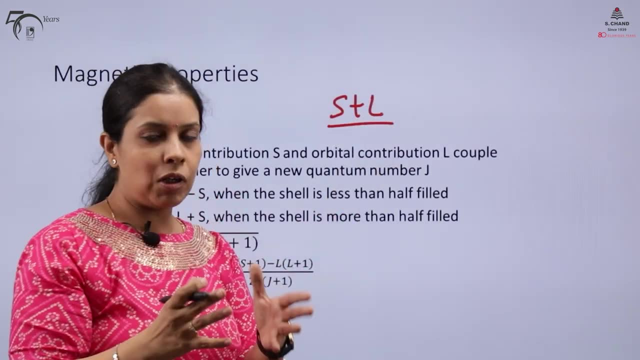 Right, There is no quenching, So we will use this. And in fact, sometimes what happens is, as we had told you, spin-orbit coupling happens, So S plus L are coupled in each other And we make a new quantum number, J. 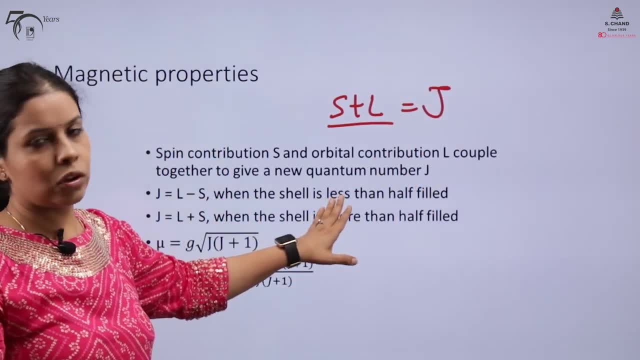 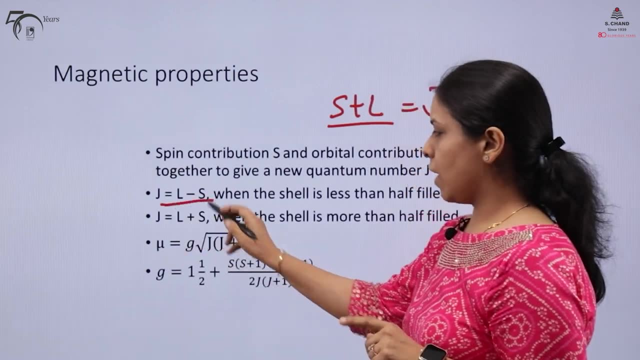 So how do we remove this J? We take two criteria in this. When the shell is less than half filled, it is shown as J is equal to L minus S, And when the shell is more than half filled, it is shown as J is equal to L plus S. 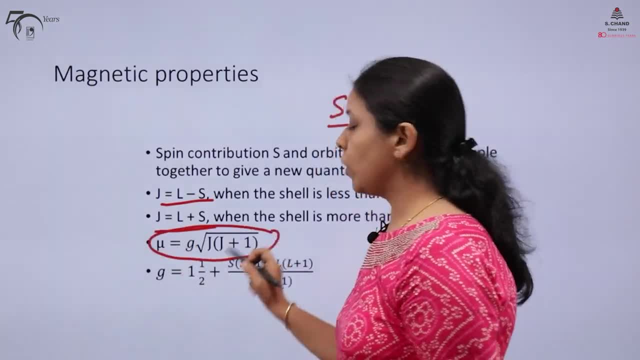 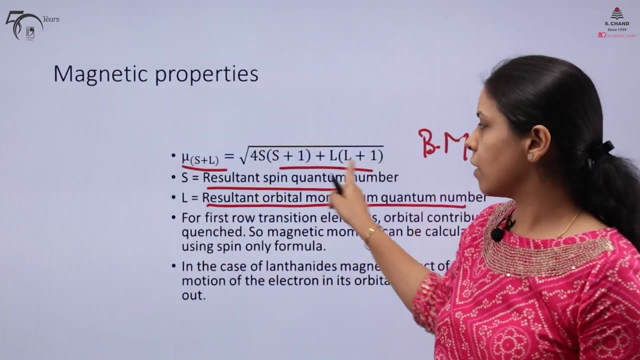 So we use J in this formula when spin-orbit coupling is taking place. When spin-orbit coupling is not taking place- we have seen the formula in the previous slide, which we have seen it like this: We will use this to remove the magnetic moment. 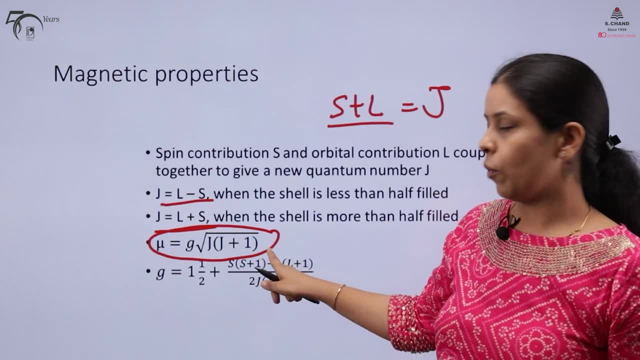 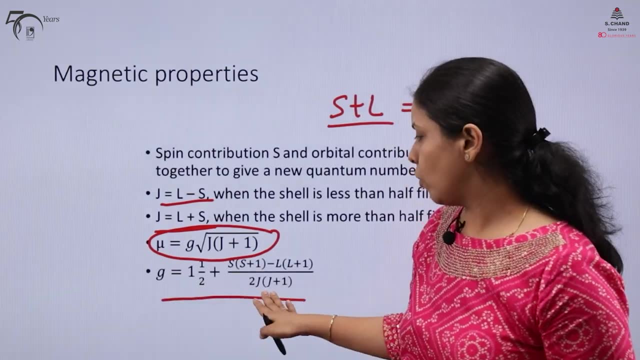 And when spin-orbit coupling is taking place. in that case we will use this formula. So, over here, G is your land-age G factor, which is calculated like this. So by removing this formula, we will remove the value of G. 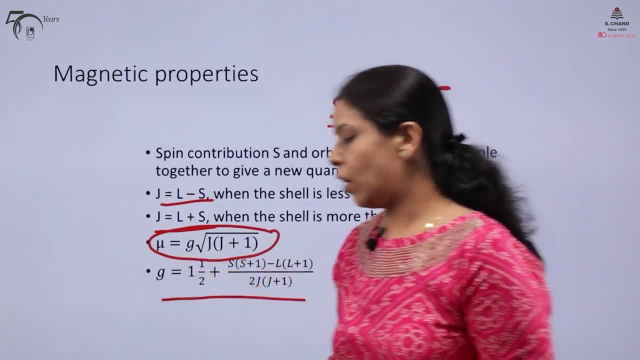 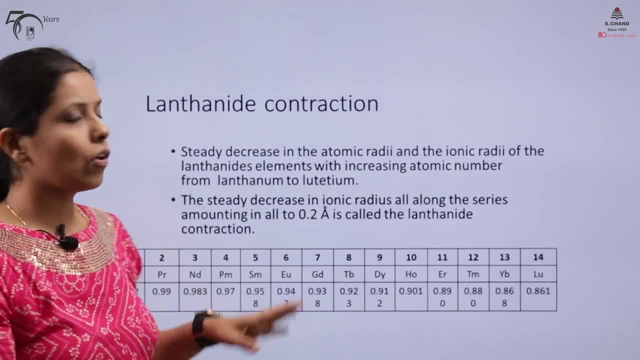 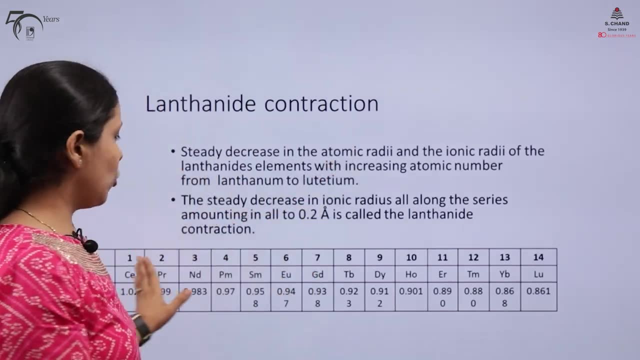 I hope this is clear to you all. So let's move ahead. So this is also another very important topic: lanthanide contraction. What is lanthanide contraction? You all know that when we are going from left to right in a periodic table, 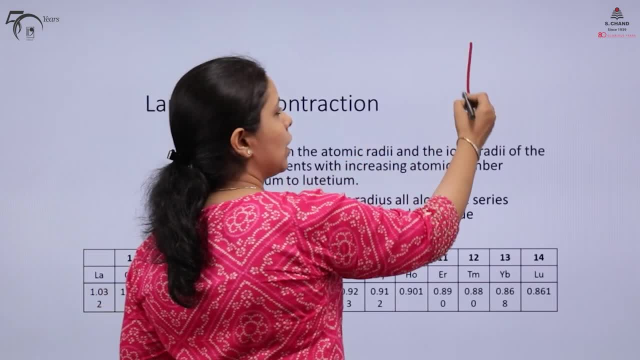 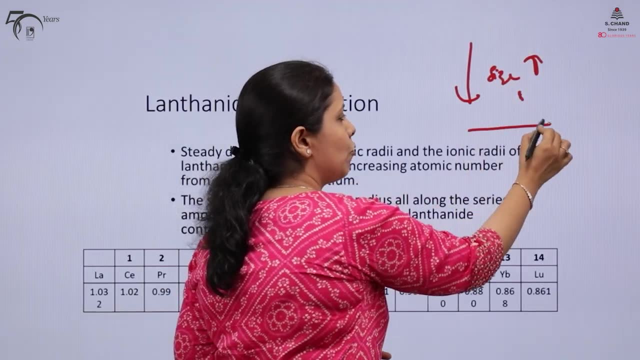 one by one. you know that when we come from top to bottom, a whole new shell comes, So our size increases, right. But when we are going from left to right, one by one, a proton and an electron are added. The proton is going to the nucleus and the electron is going to the orbital. So if the electron that is going to the nucleus cannot be shielded properly, then the proton will attract it And in that case your size will decrease. 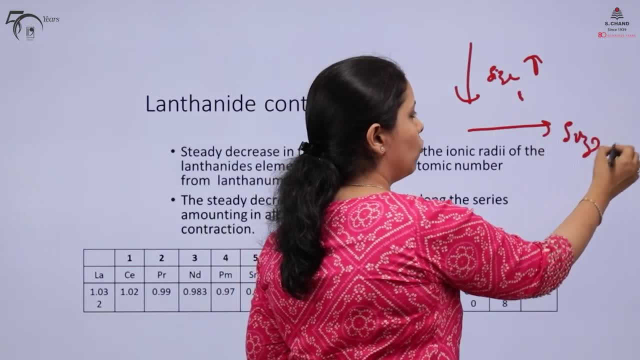 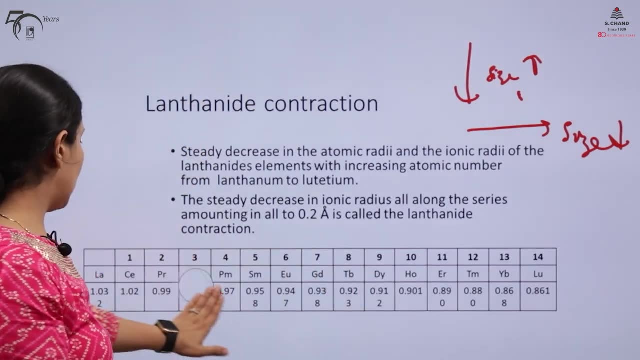 So when we go from left to right, the size decreases right. Similarly the case with the lanthanides. Now we have taken only lanthanides. So what happens in lanthanides Our When we are filling this? 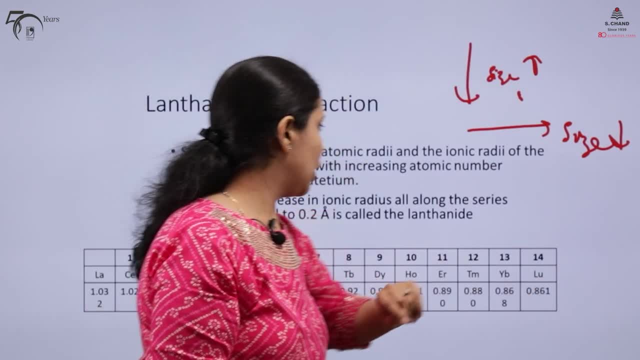 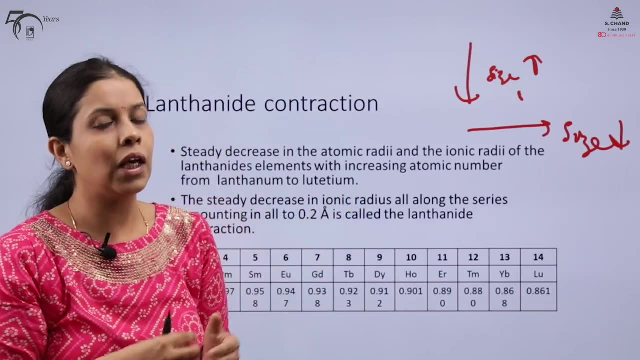 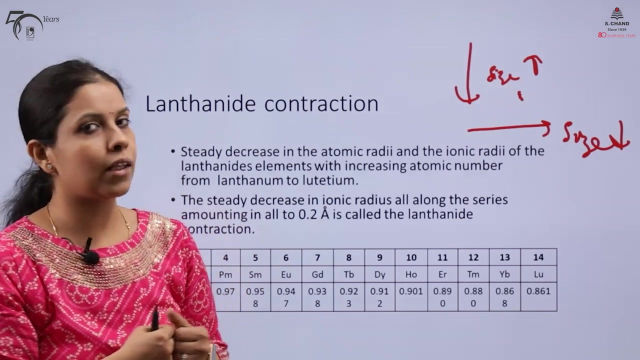 we are filling this electron in the F orbital from cerium to lutetium. So the screening effect of the F orbital is very less because they are very diffused So they cannot be screened properly. So in that case your protons in the nucleus attract it. 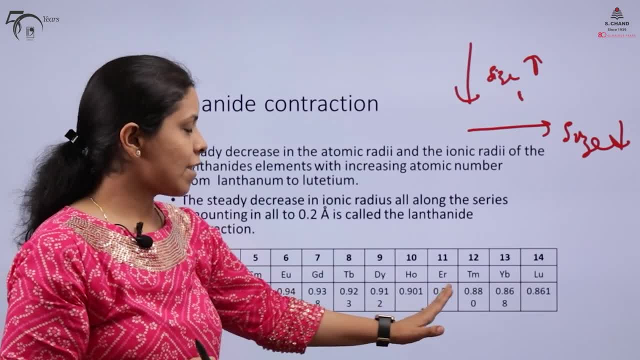 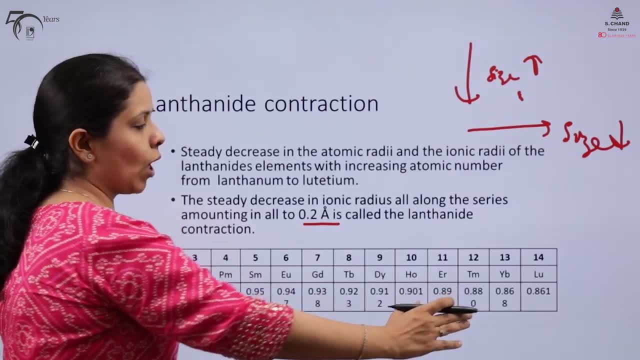 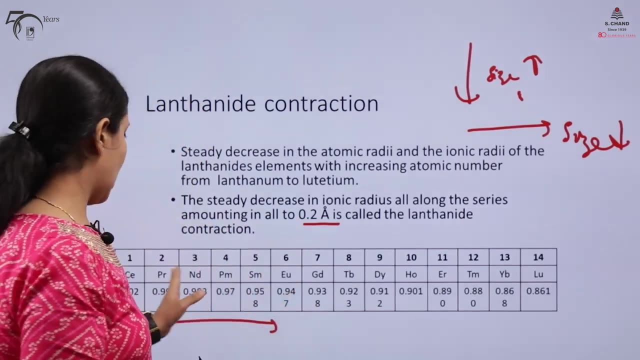 and your size decreases. So a study decreases in size which results in a total of about 0.2 angstroms, And this decrease, which is observed in the whole series, is called lanthanide contraction Right, So these are known as lanthanide contraction. 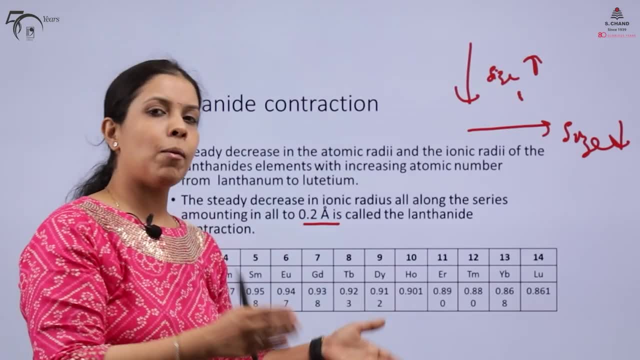 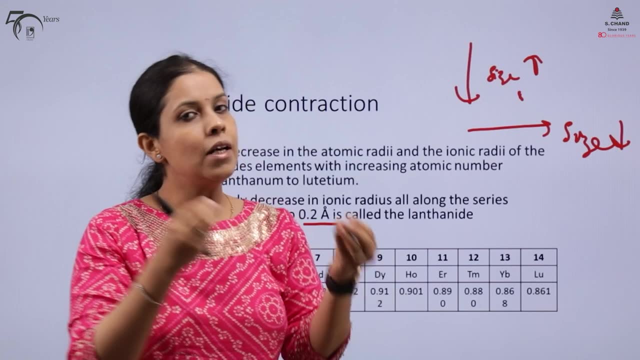 which we observed in the lanthanide series. Similarly, when you study actinides, there will be actinide contraction also. So as the size is decreasing in the lanthanide when we are going from left to right, similarly the size decreases in the actinide. 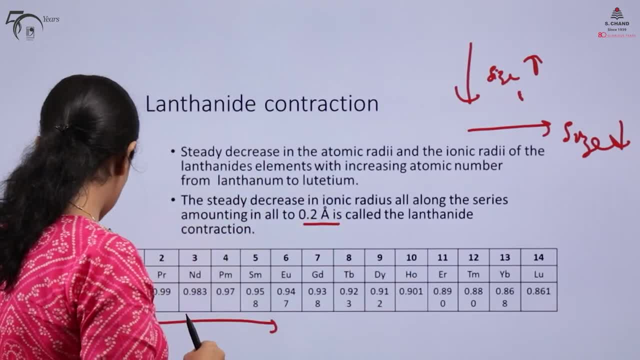 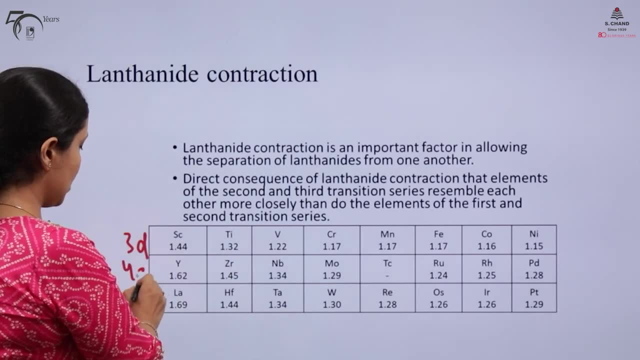 when you go from left to right, Right, So the terms are same. Now, what is the effect of this? This is our 3D series, 4D series, 5D series, Right. These are all your transition elements. 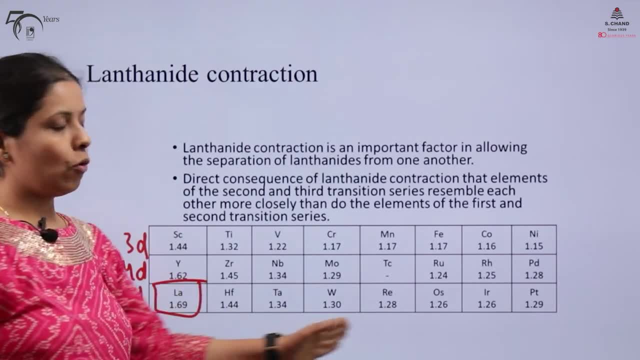 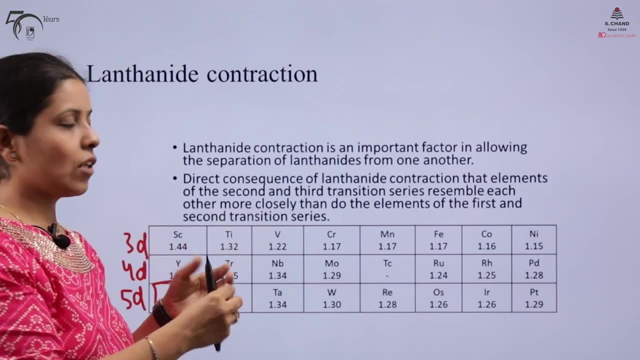 So you know that after lanthanum your whole 4F series has come. 4F orbitals are filling And because those 4F orbitals, due to your lanthanide contraction, the size has decreased, So you will get the effect of them. 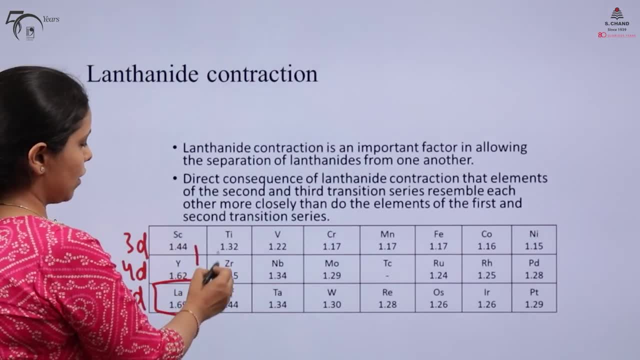 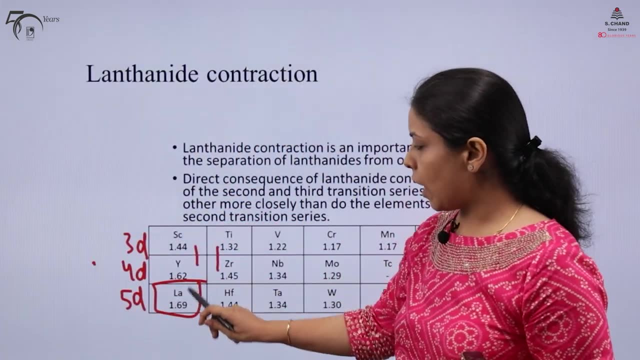 in the transition elements also. Now you see, when you go from 3D to 4D, the size is approximately increasing, Right, But when you are going from 4D to 5D, as you came from here to lanthanum, 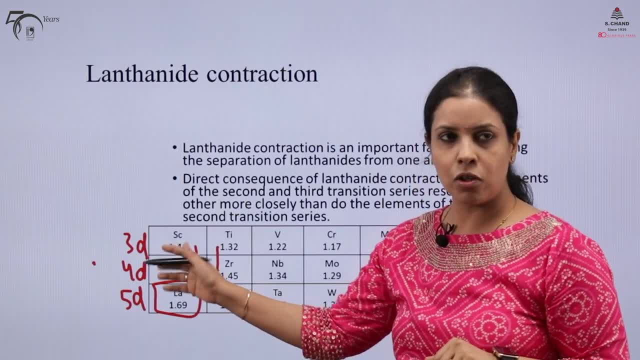 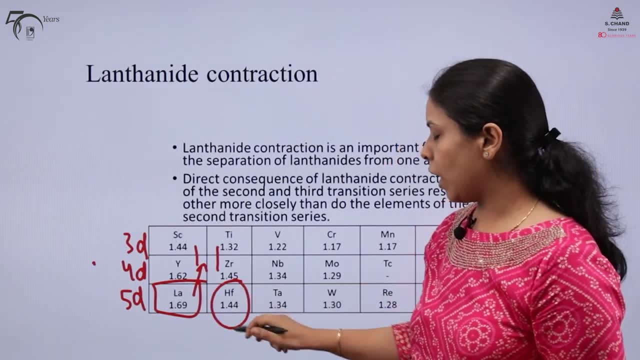 then the size is increasing here, which should be because you are coming to the next orbital, But after lanthanum your whole 4F series has filled. So when you have come to hafnium, then the size has not increased. 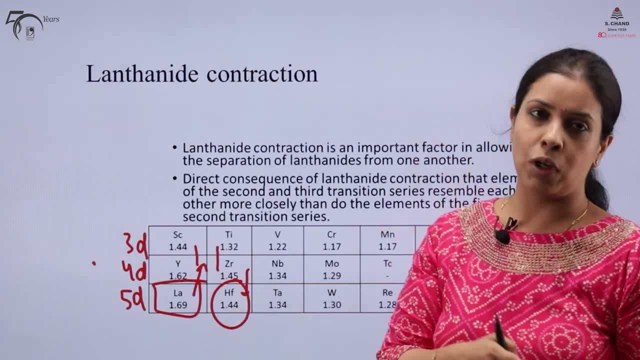 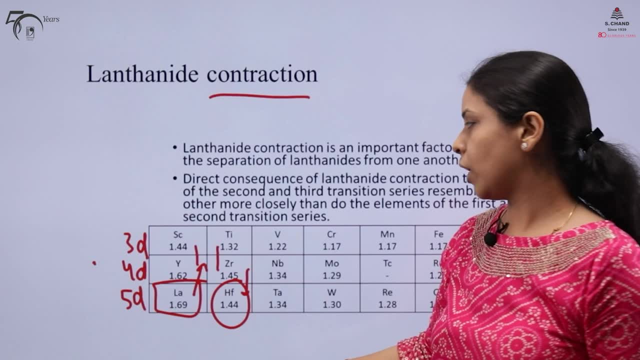 from zirconium to hafnium. In fact, the size has decreased, which is the effect of lanthanide contraction. So this is the effect of lanthanide contraction, which you will get to see in the transition series. 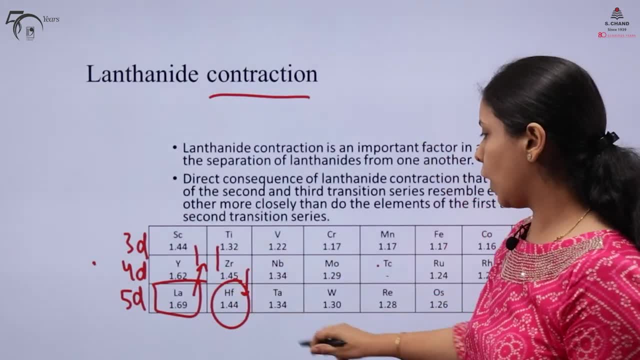 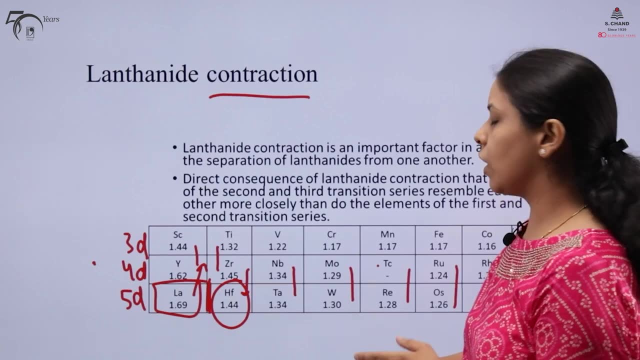 In 3D and 4D the size increases. But if you see after this, because here all your lanthanides have filled, then after that your size should not increase in the orbital. So because of this, 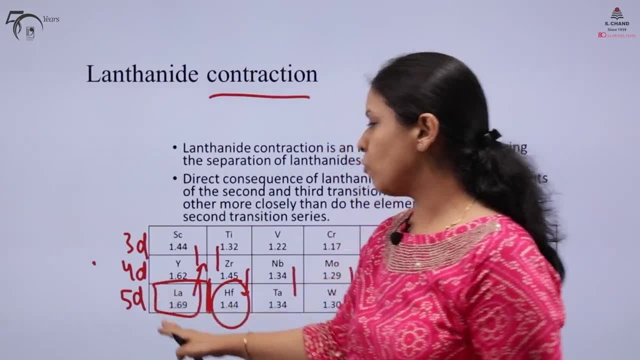 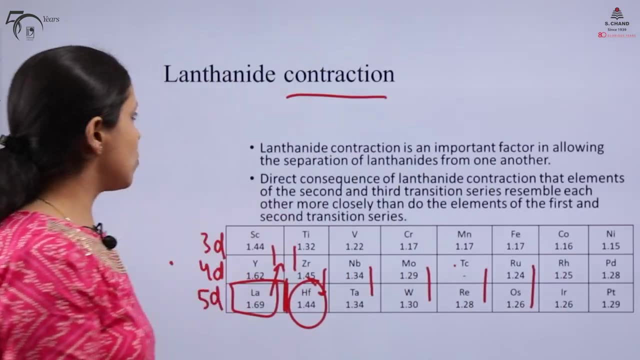 the properties of 3D and 4D are different, But the properties of 4D and 5D they are more or less same because their size remains same. This is the consequences of lanthanide contraction. Next topic: 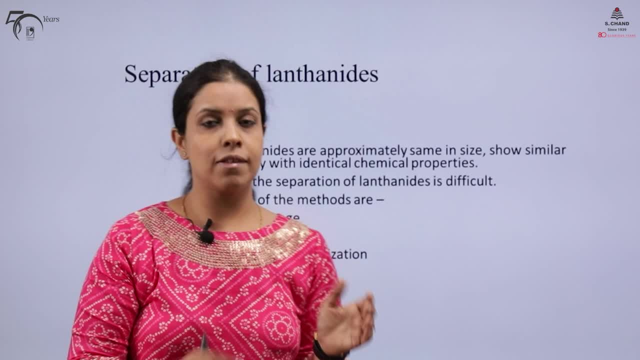 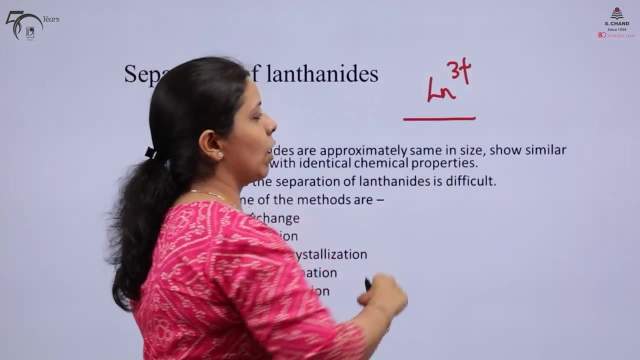 which we are going to discuss in today's video is separation of lanthanides. Now you know. I have told you what is the most common oxidation state of lanthanides. It is plus 3.. The size of lanthanides is also same. 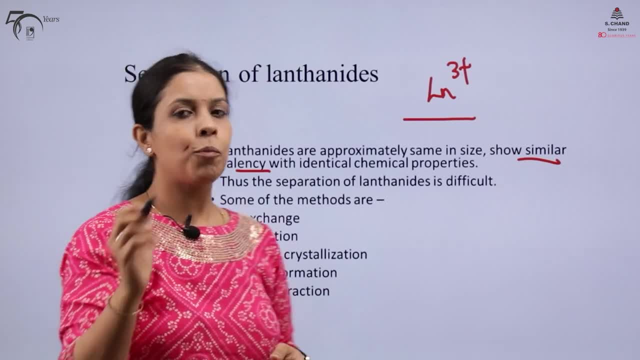 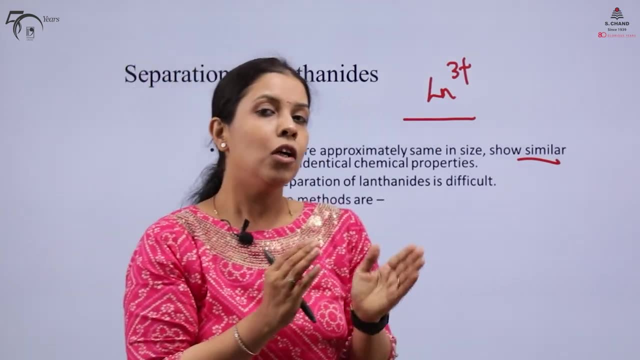 So they are showing the similar valency, Because of this, their properties, which obviously depends on them. what is the size the variable oxidation state is showing or not? so their physical and chemical properties are also same. There is not much difference. 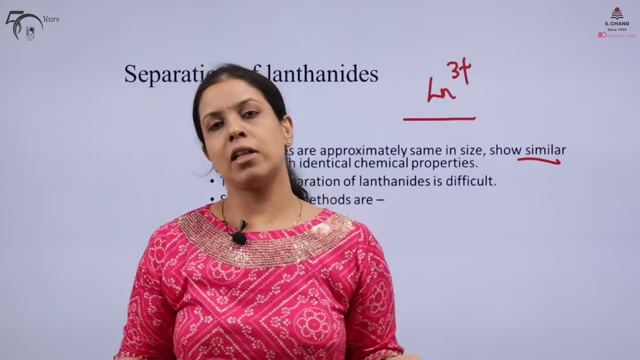 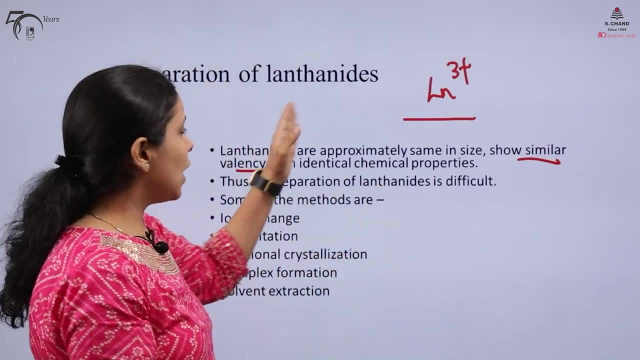 So when you want to separate a mixture of any compound, then you see these properties, that some of their properties are different, on the basis of which they can be separated, But in the case of lanthanides, this is not the case. 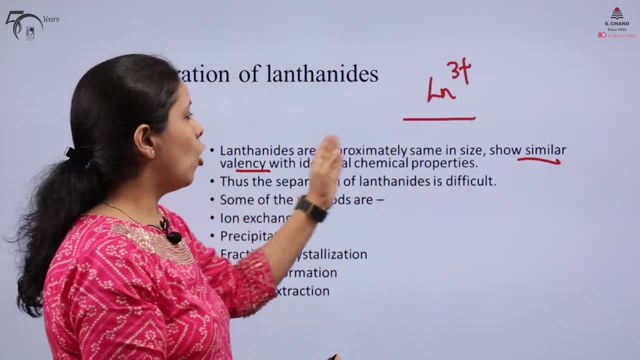 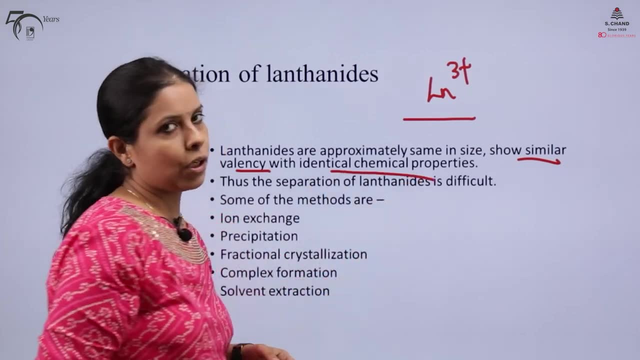 because the charge of ions is same. almost the size is same. so because of that, atomic radii and ionic radii are almost similar, because of which their properties are same, So it is very difficult to separate them. 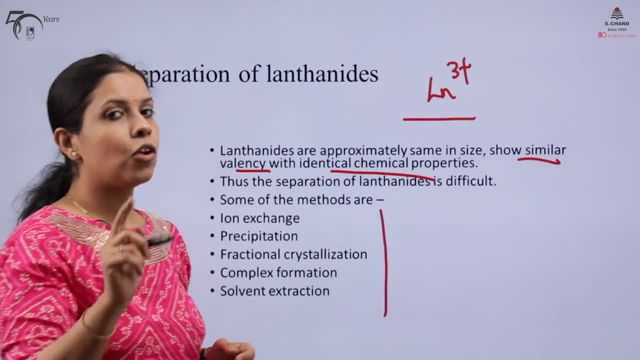 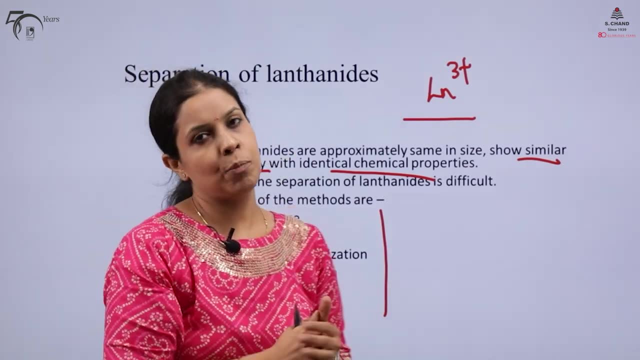 But still we have some of the methods by which we separate lanthanides, because lanthanides mostly exist in the mixture, naturally, So it is very important to separate them. If we want to use only one lanthanide particularly, we cannot use the mixture. 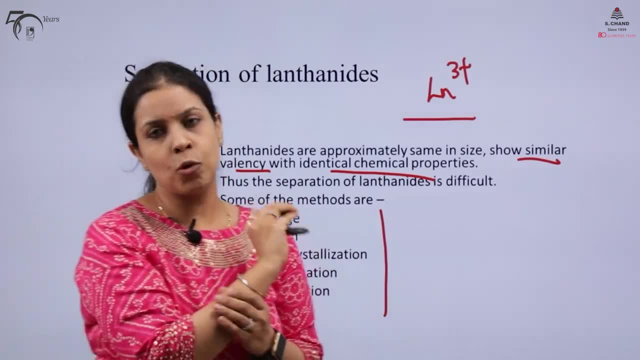 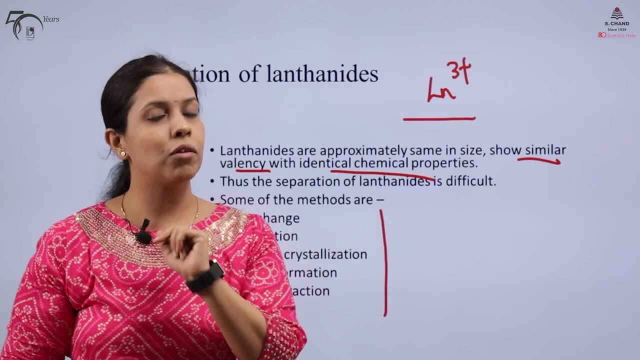 In fact we need that particular lanthanide in the as purest form as possible. So we need it in the pure form. So we have to separate the lanthanides, But their separation is very difficult, So we have some methods. 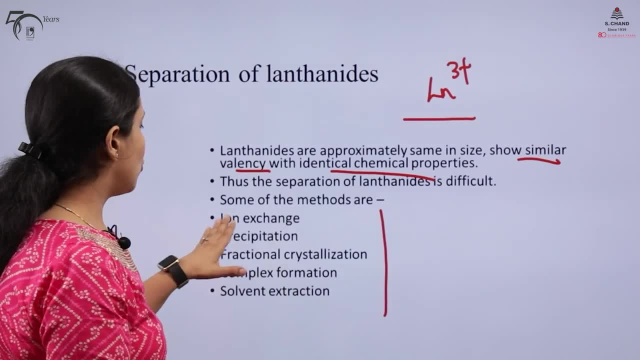 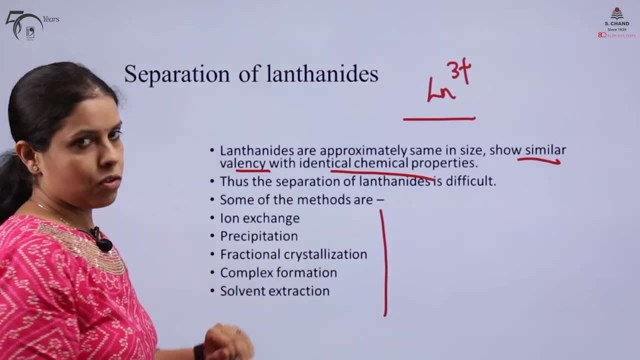 which we use for having the separation of lanthanides. So those are: ion exchange, precipitation, fractional crystallization, complex formation, solvent extraction. So we have a lot of methods, But in today's video we will discuss only one method. 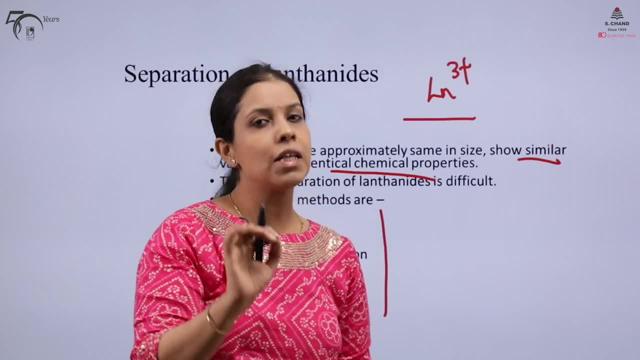 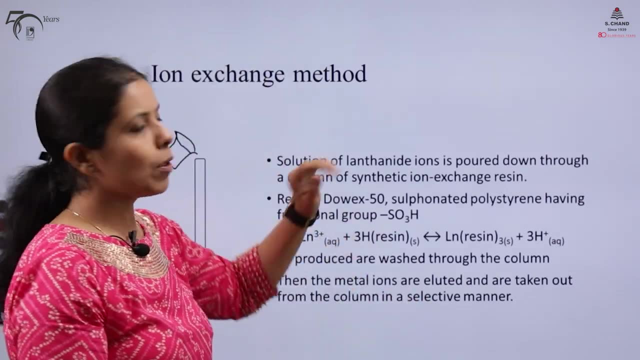 ion exchange, which is the most common and the easiest method to separate the lanthanides and to get the pure lanthanides which we need. Now what do we do in ion exchange? So we take such a column and fill it with resin. 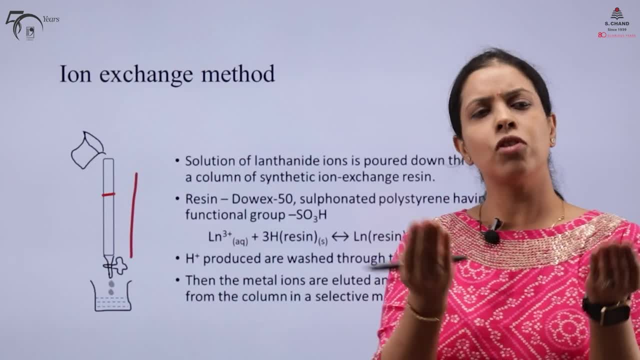 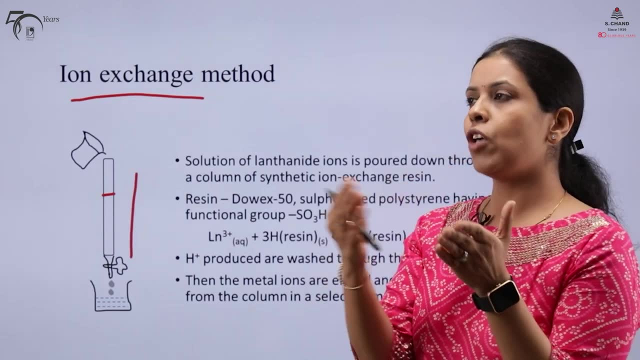 Resin is a solid, straight formed resin which contains some cation or something like that, which can be exchanged. That is why we call it ion exchange, because in resin there are some free charges which you can separate and later you can elute it. 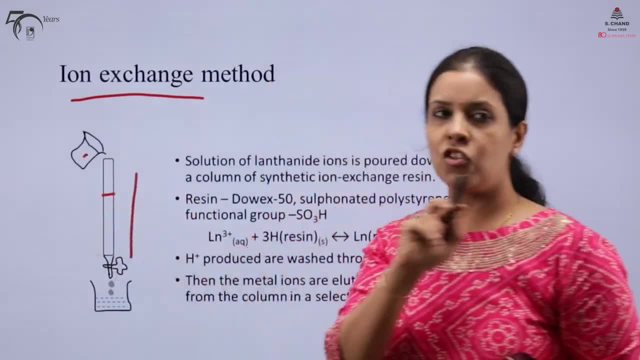 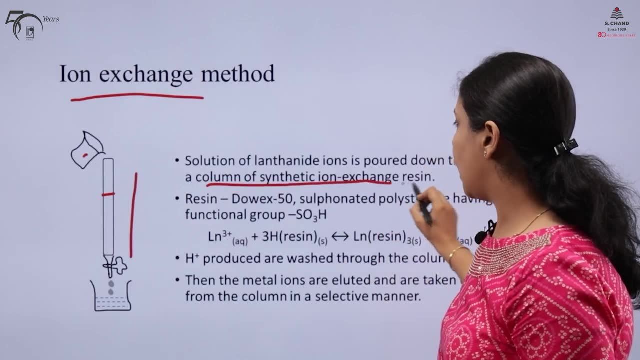 So what did we do Here in the beaker? we took a mixture of lanthanides, which we have to separate. Right Solution of lanthanides ion is poured down through a column of synthetic ion exchange resin. So this is the resin. 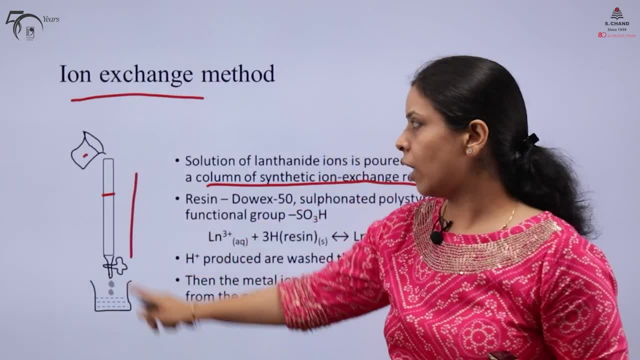 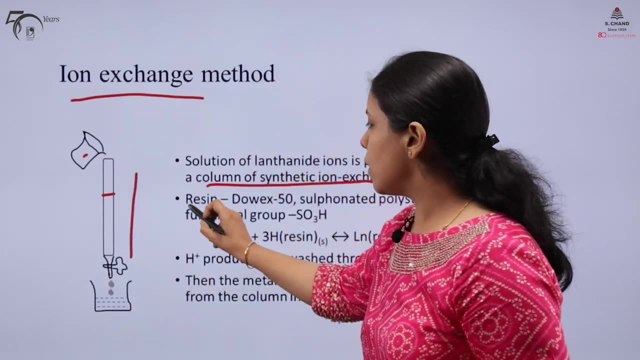 which we have filled in this column, which is in a solid state, And we have taken the solution of our lanthanides, which is obviously in liquid form. So when we poured it, the resin which we usually take is Dovex 50.. 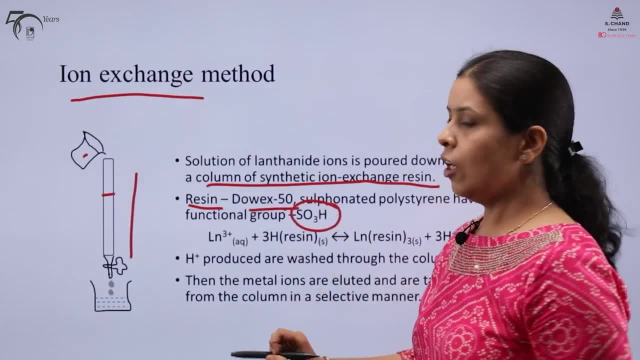 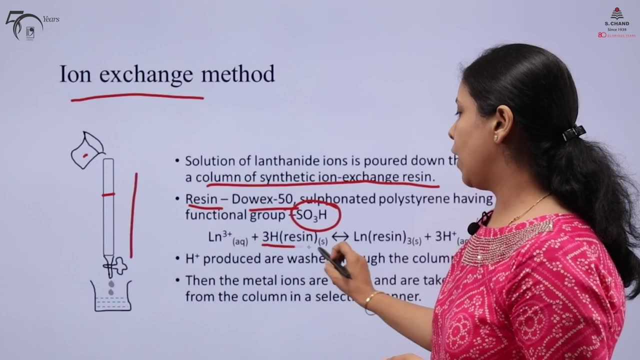 Okay, So the functional group in it is SO3H, So its hydrogen ions are free. They are exchanged with any ionic species. So this is our resin, in which H plus ions can be exchanged easily. Lanthanide is 3 plus ion. 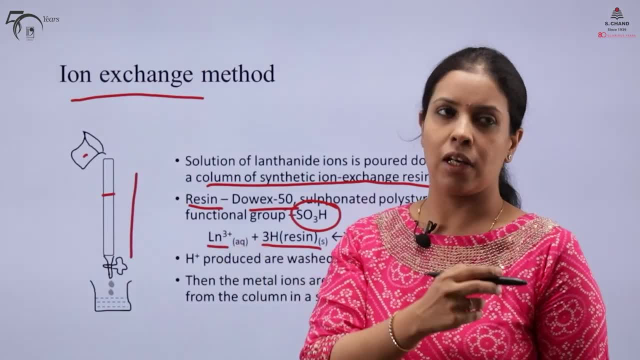 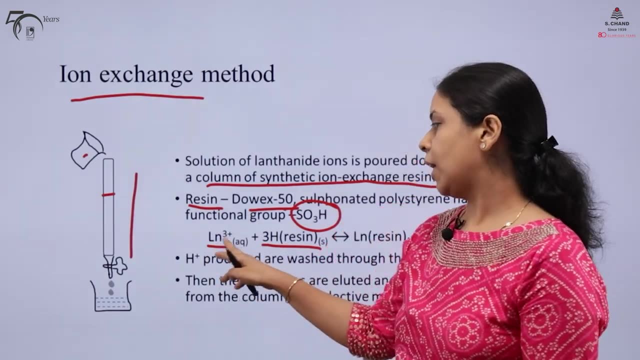 That is why I have written Ln 3 plus, because it is a mixture. Ln is represented for lanthanide. There is no lanthanide. This mixture is represented by lanthanide. So when we have poured the mixture of lanthanide. 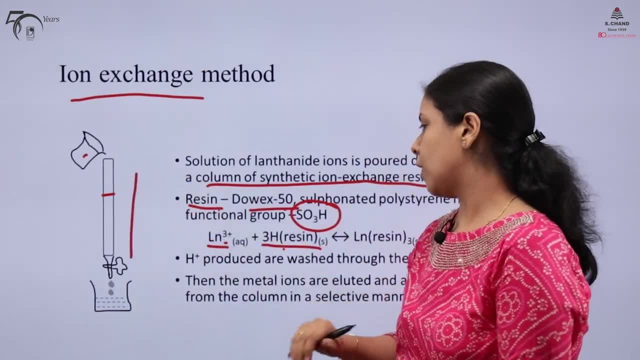 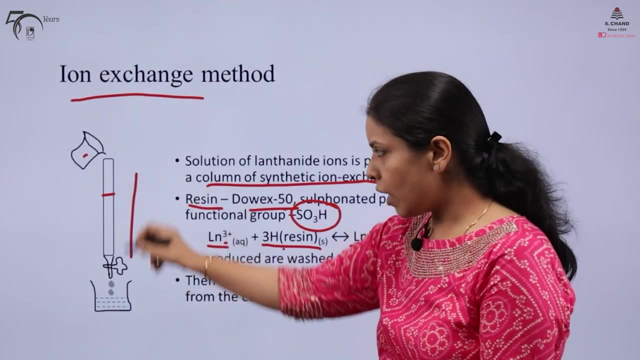 from above and in this column we have this resin. So the H plus of resin will be exchanged. And what will come on the resin? Lanthanide: Because our resin was in solid state, We have poured the mixture of lanthanide. 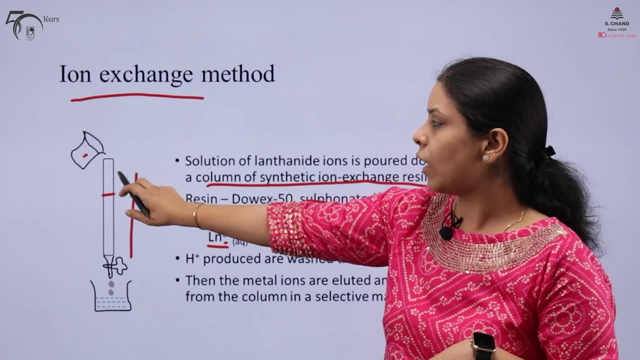 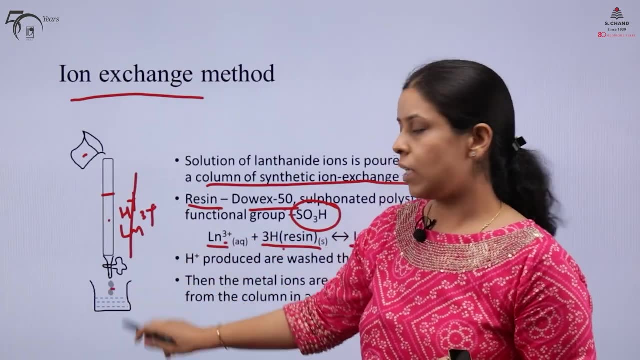 from above, which is in liquid form. So what happened now? In this solid state, our lanthanides have come in place of H plus ions. Right, And what will come in the lower solution? H plus ions. So we can take out. 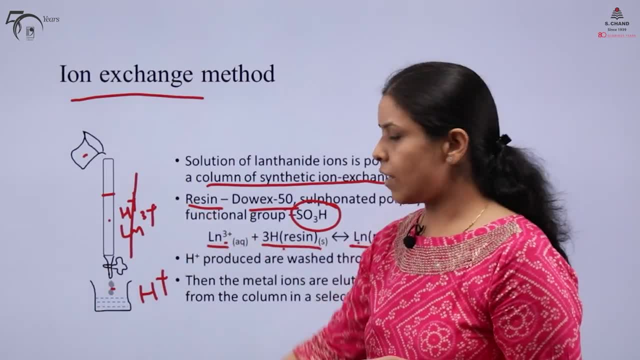 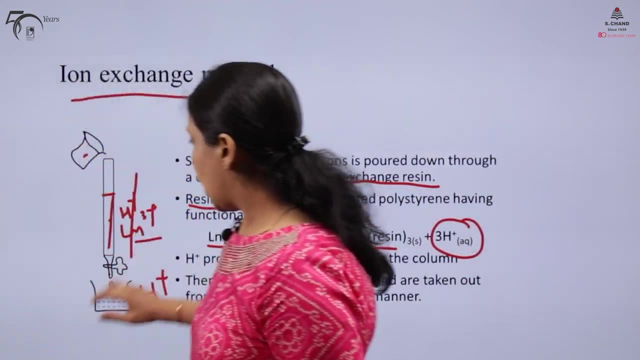 H plus ions. There is no problem. We have taken out H plus ions And in this resin we have now Ln 3 plus. Right. So now? what is our problem? Now we have to take out Ln 3 plus. 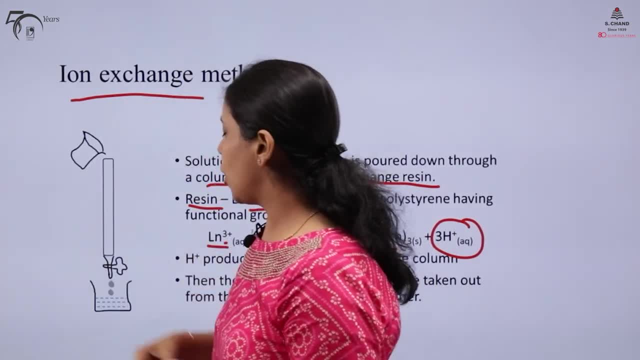 Now, how will we take out Ln 3 plus? Now in the mixture, our Ln 3 plus has come, So now, how will we take it out? So now these metal ions are eluted and are taken out. 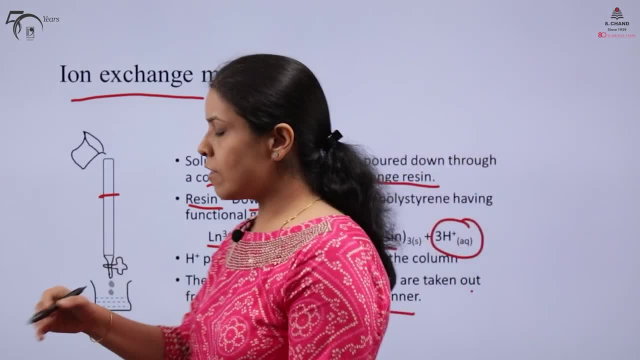 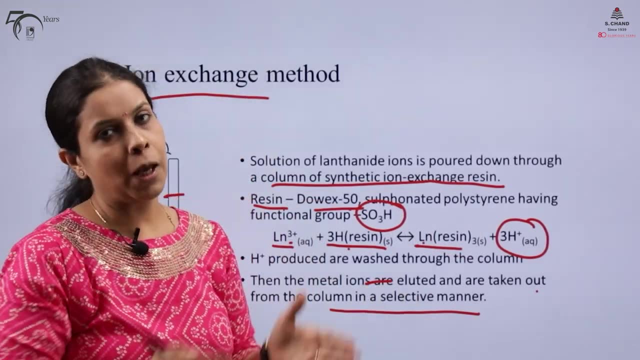 from the column in selective manner. Now we have, suppose, two or three or four mixture of lanthanides that we had put in. All of them have stuck with our resin. Now we have to take it out selectively so that 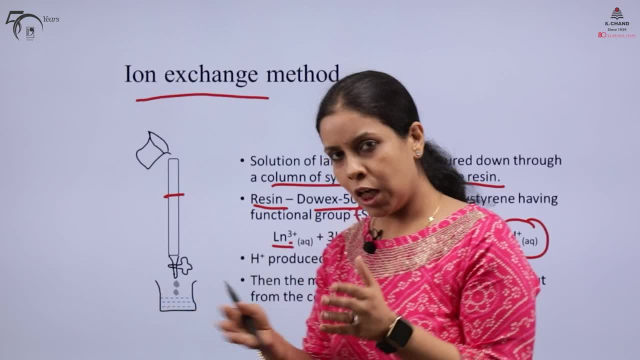 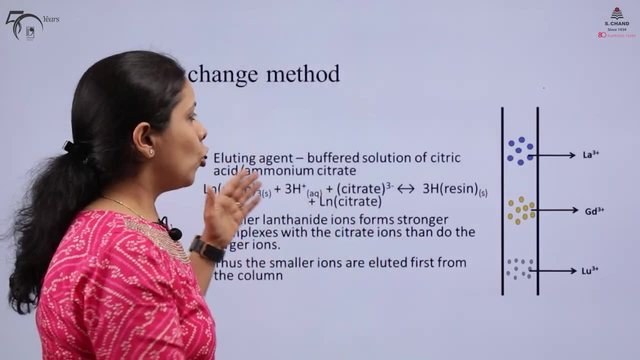 as it comes out. it can be removed or it can be selected in our different forms. So what will we do now? We will take an eluting agent. To take out anything means to elute it, So the agent that we use- 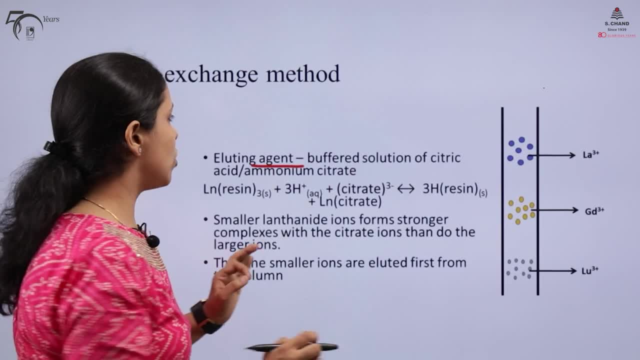 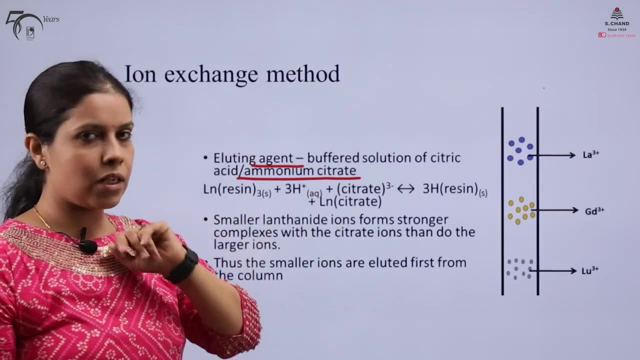 is called eluting agent. So the most common eluting agent which is being used is buffered solution of citric acid or ammonium citrate. Right, So we use this solution as an eluting agent. So we have in resin solid state. 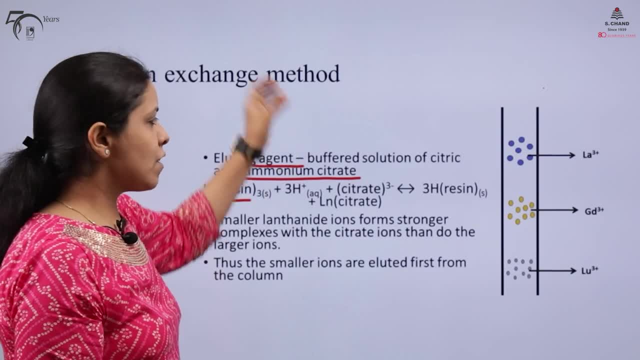 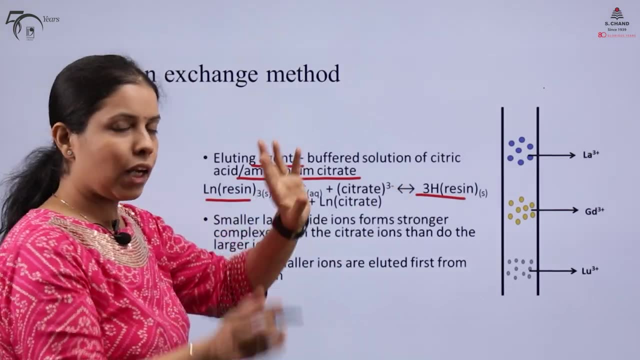 on which lanthanides have gone. Now, if you have poured citric acid in your solution in the column, then our H plus again came to the resin which was there previously, which had been exchanged with lanthanides. Now a complex has been formed. 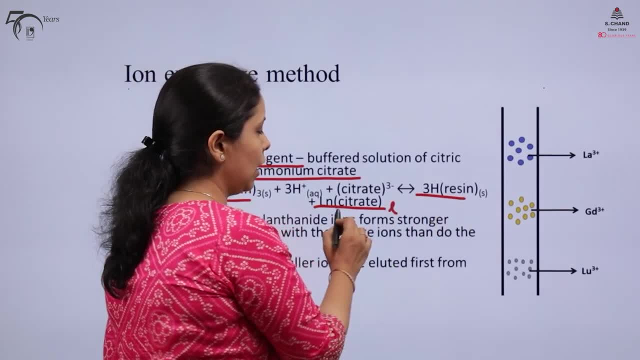 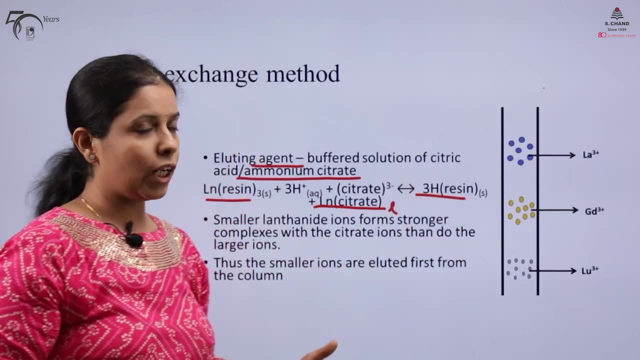 lanthanide citrate. This is in, this is solid now and this is liquid Right. So now this is in aqueous state. Now this lanthanide citrate complex will get removed from the column one by one Now. 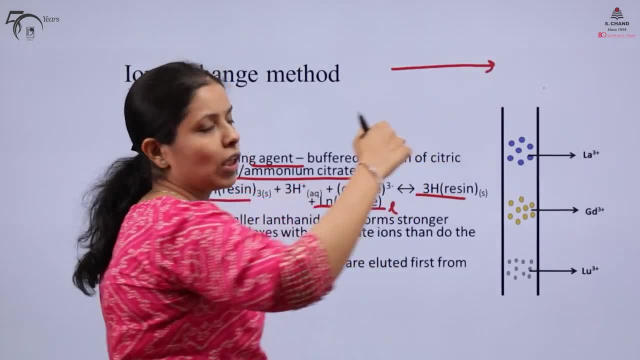 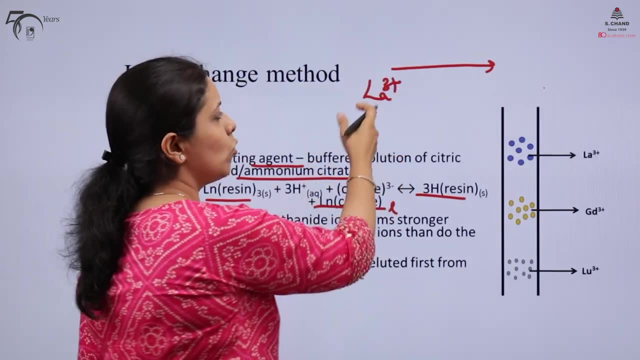 what is the property which will separate it? Let us go to right side. Size decreases, So the biggest one. for example, if we include LA3, lanthanum 3 plus, then it is the biggest, and Lutatium 3 plus. 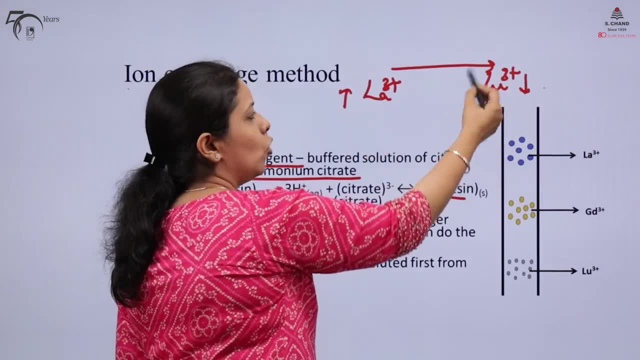 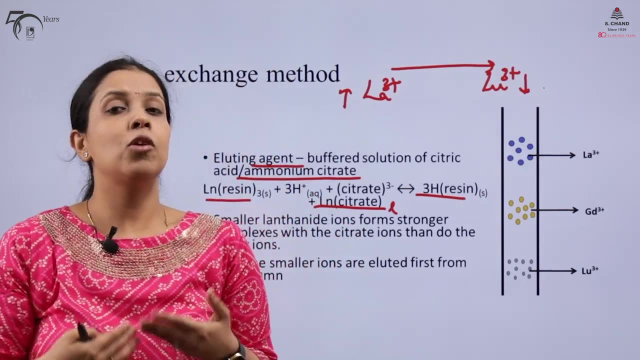 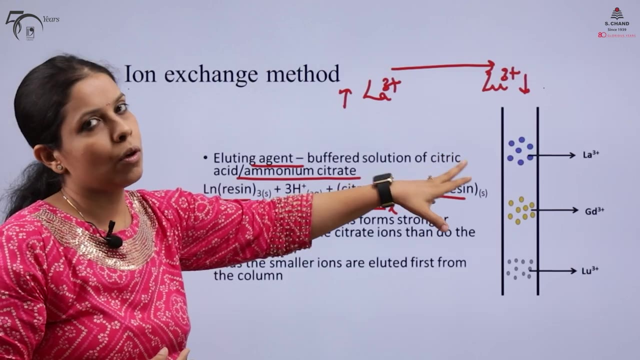 is the smallest in size. So this is the smallest and this is the biggest right Size wise. So Lutatium 3- now you know the size of metal- is small- it can make a better complex. Its complexing ability, ability to form the complex. So Lutetium will make the best complex. The better the complex will be. 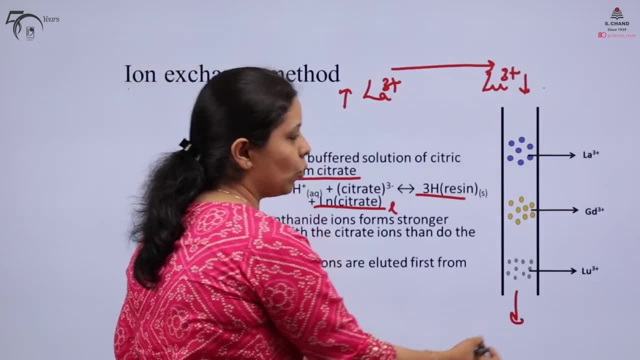 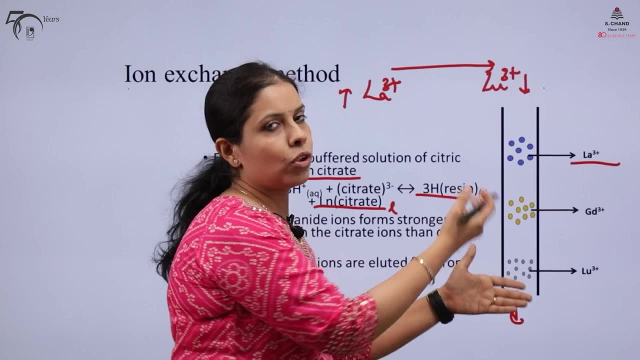 the faster it will come out. So Lutetium will be elute first and Lanthanum later. So if there is anyone in between whose size is obviously in between these two, then according to that we can collect it. So first you have eluted the smallest ion. 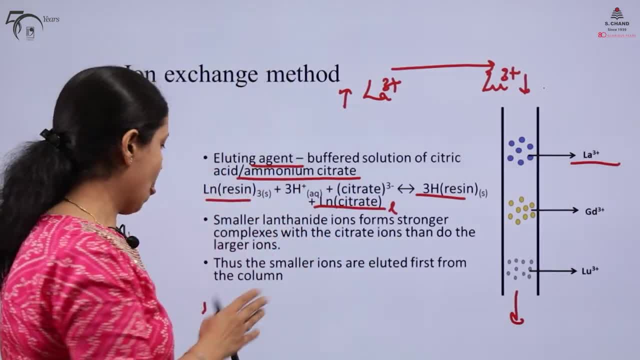 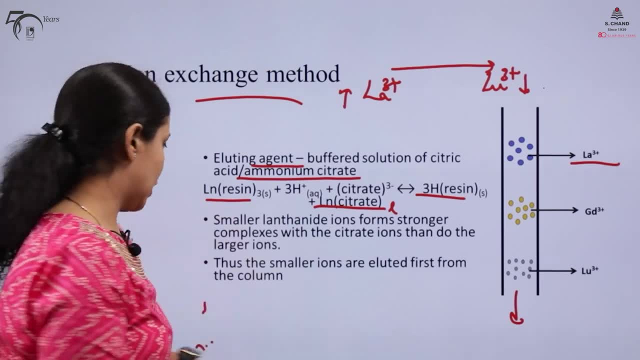 then the largest, then the largest and the largest will come later, Right? So this is the method of ion exchange which is very simplest and the most common one which are used for the separation of lanthanides. So our lanthanides are completed here. We. 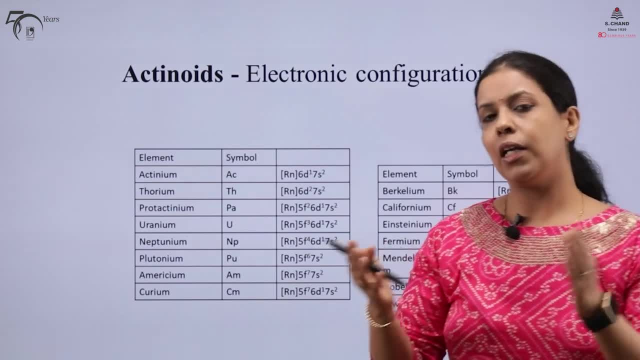 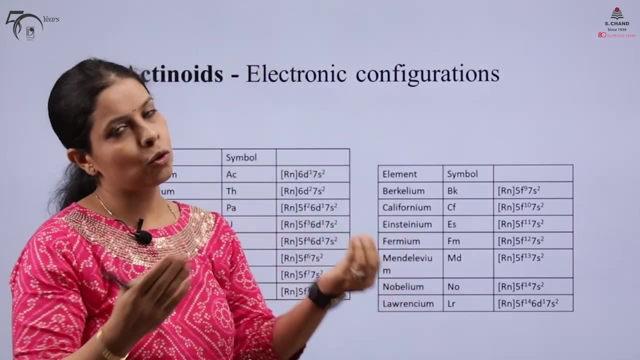 have read the lanthanide contraction. we have read its atomic radii. we have read the electronic configuration. Now we will read some actinides. Many properties of actinides are same as lanthanides because both are F-block elements. Both have 14 elements. I have already told you that after. 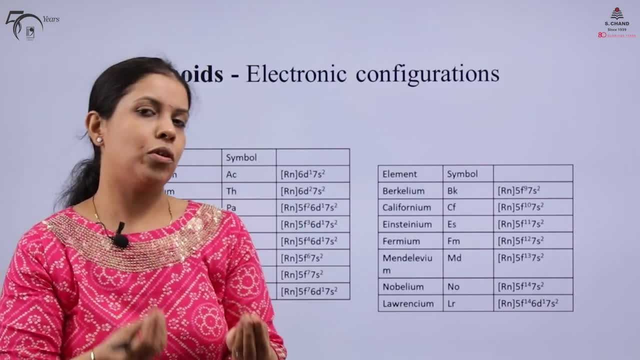 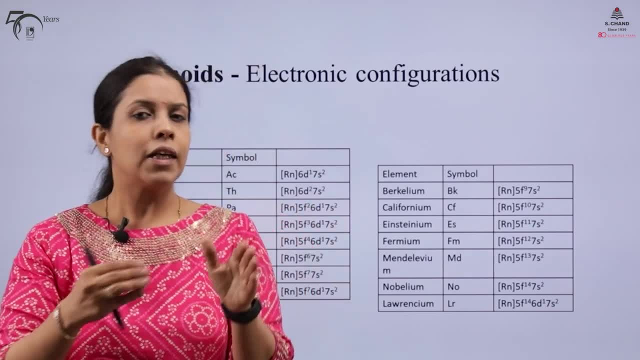 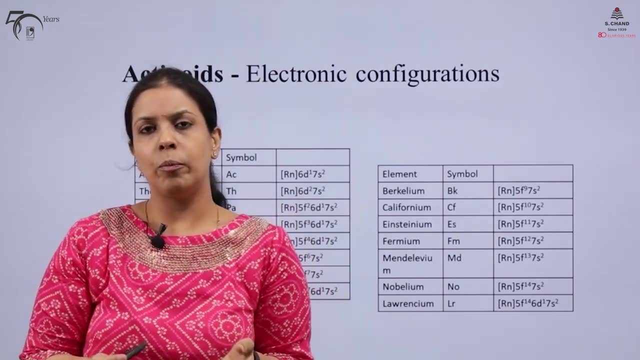 are actinides. Most of their properties are actinides. The properties of actinides, or let us say that they are same as lanthanides, such that their spectra was the same and then their oxidation state was plus three common. so they and you. 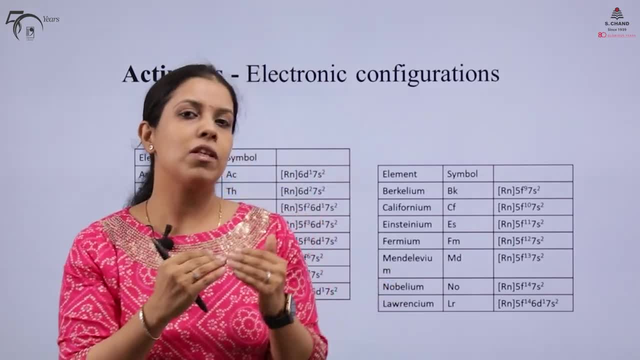 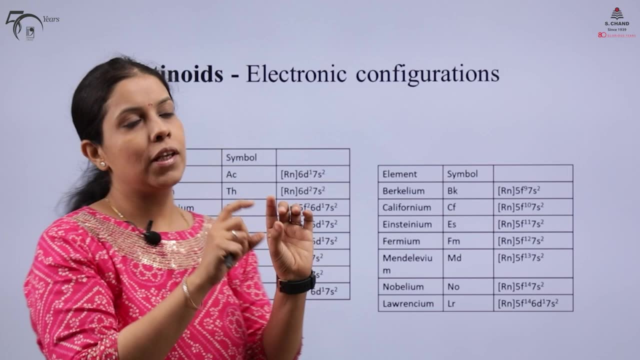 know those who come in one group. Their properties are similar. So, oder based on these Parameters, all our actinides have been placed under lanthanides, and this is how it has come up with a 5F series with 4F, which we call as actinides, Right. So? 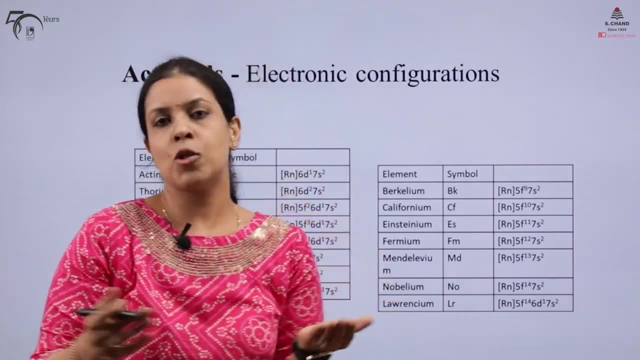 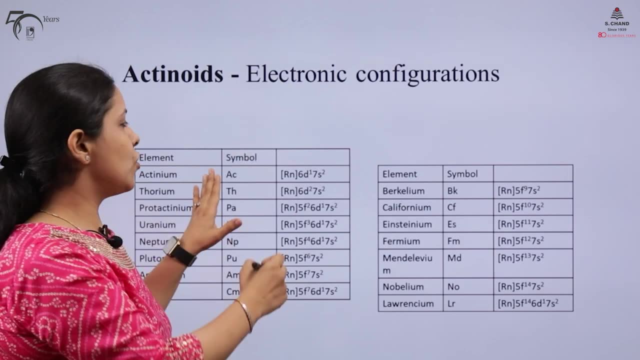 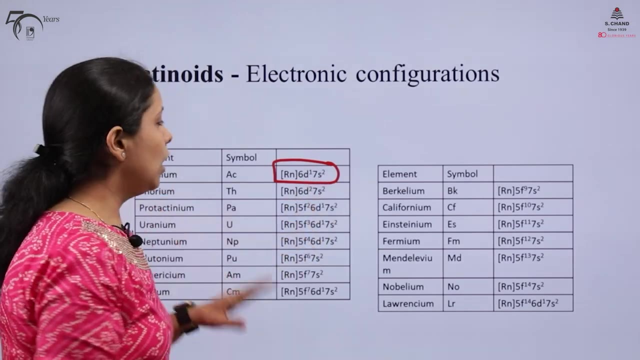 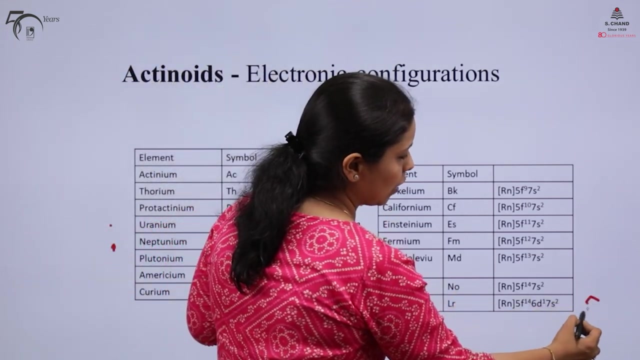 configuration is very important for us to understand, on the basis of which you can discuss other properties. so we will discuss this. actinium is our transition element, where you have redon noble gas configuration. after that, 6d1, 7s2 comes now, as expected. what you should have is that here from 5f1, you fill the entire 5f14, because there are 7 orbitals, so 2 electrons will go in each, so total 14 electrons will be filled. 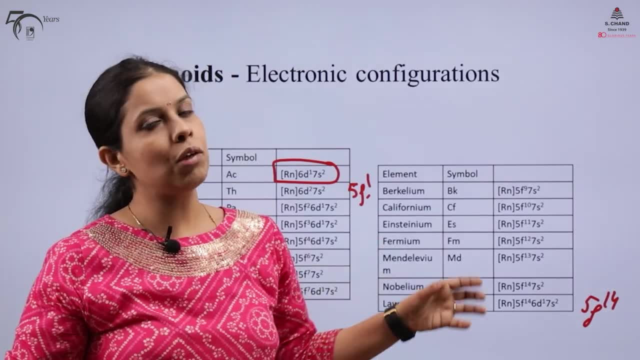 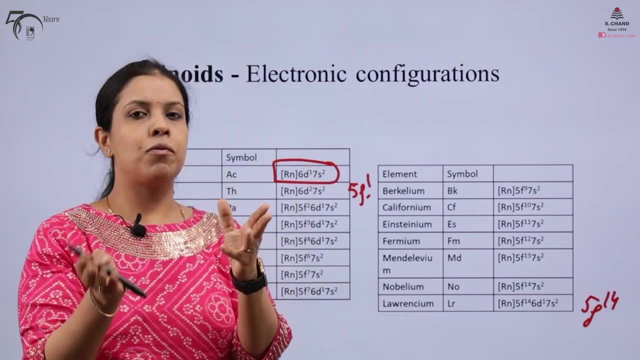 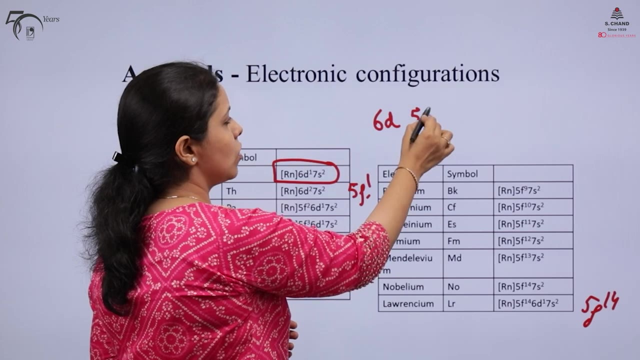 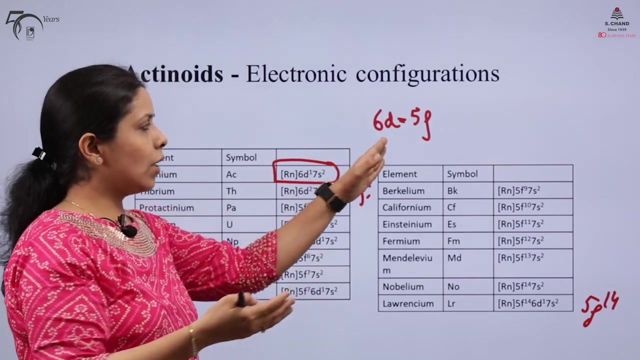 and our 5f series of actinides will be totally filled. but you know, in the case of lanthanides we discussed that what was there? 4f and 5d and 6s energy was same. what happens in this too: usually 6d and 5f energy is almost same. so sometimes, to give more stability to that particular element, the 6d electrons come in 4f, like in this one. 6d2 is the state. 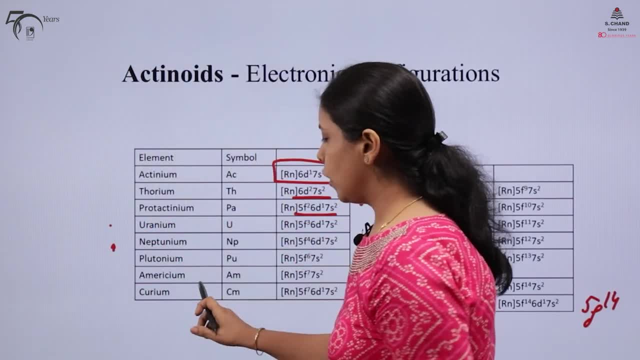 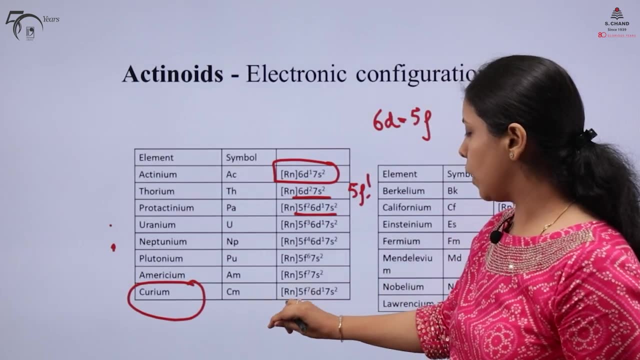 over here. it is like this over here also, like our. gadolinium was there, in which half filled orbital stability was there. over here also, curium is there, in which your configuration is 5f7,, 6d1 and 7s2,. 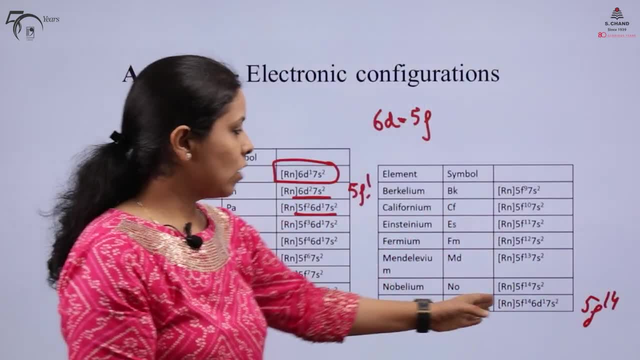 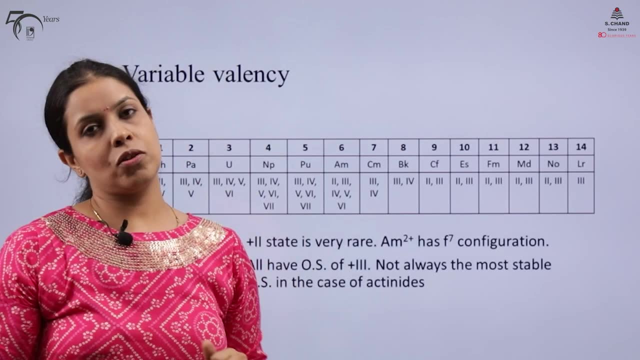 so this is half filled configuration, which is obviously more stable, and this is fully filled orbital configuration, which is more stable, mostly in the case of lanthanides. what was there plus 3 oxygen state was the most stable one. 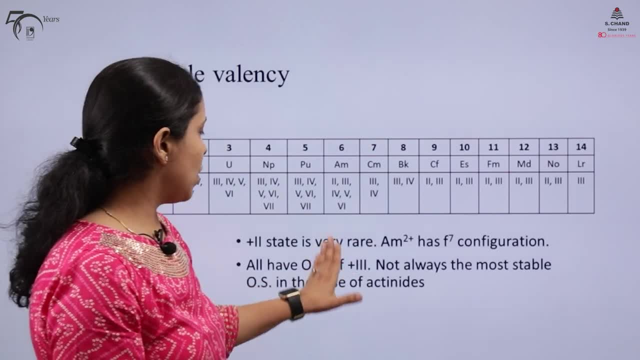 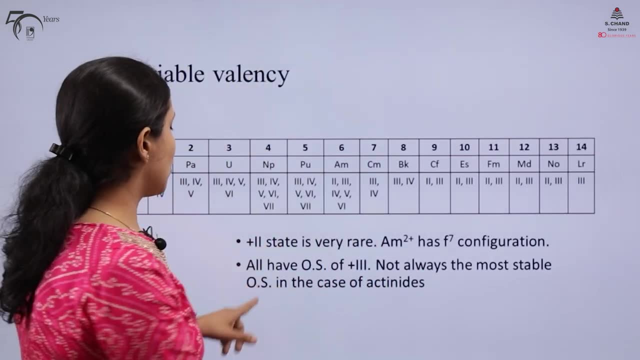 but here it is not like that. here everyone has plus 3, but it is not necessary in the case of actinide. plus 3 is the most stable right, so similarly, plus 2 is very rare. 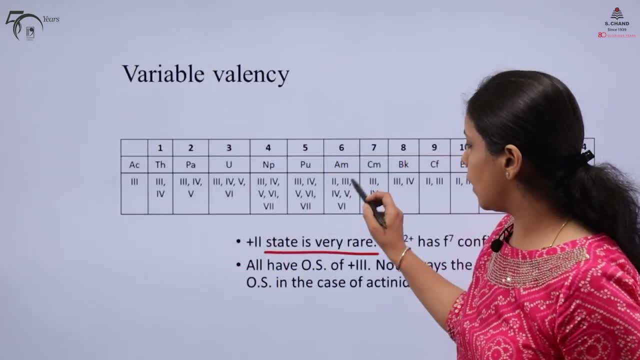 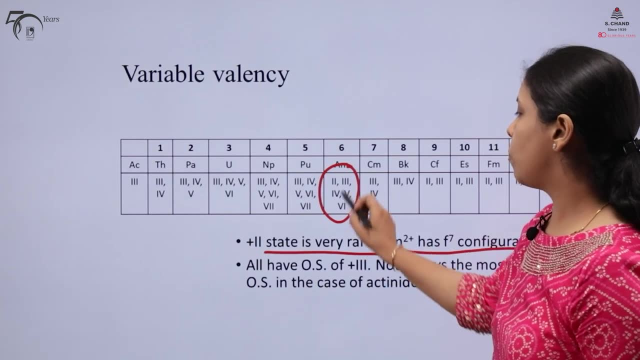 as you know, mostly plus 2 was existing in it. but here am2 plus comes in plus 2, because its half filled configuration will be done. that is why over here plus 2 is stable. otherwise plus 2 oxygen state is very rare. 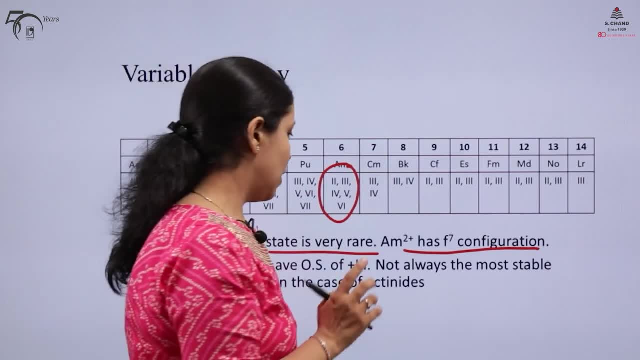 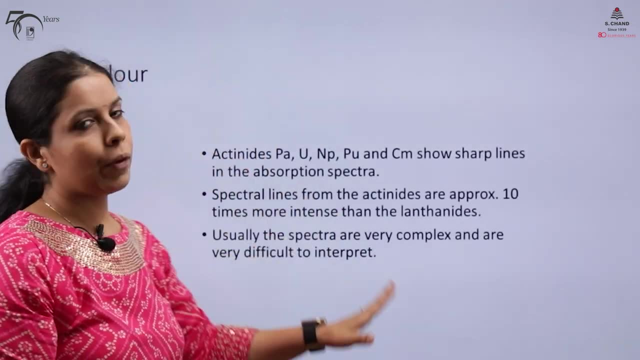 in the case of actinides as compared to lanthanides. right, ok, so next. next thing which we are going to discuss is color. color is again. you know why- color shows. we have discussed it over again and again. 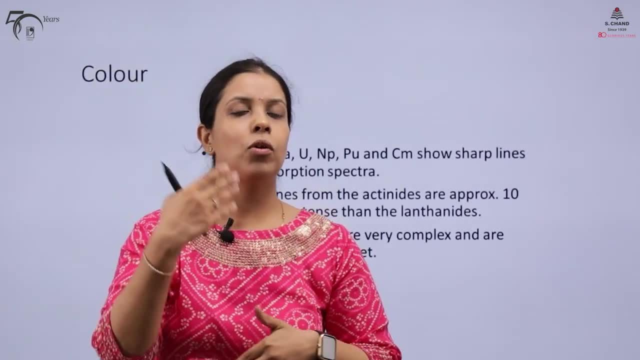 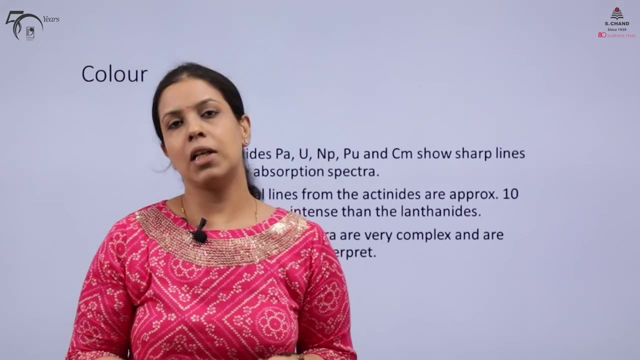 whenever there are unpaired electrons, then there is a transition in them from lower to high energy level, due to which color comes. so whenever for 5F electron in actinide series you have unpaired electrons, then 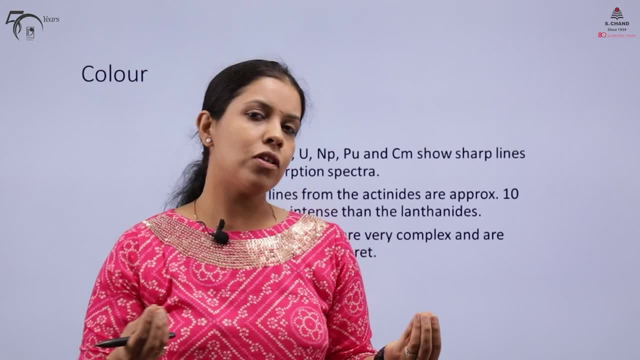 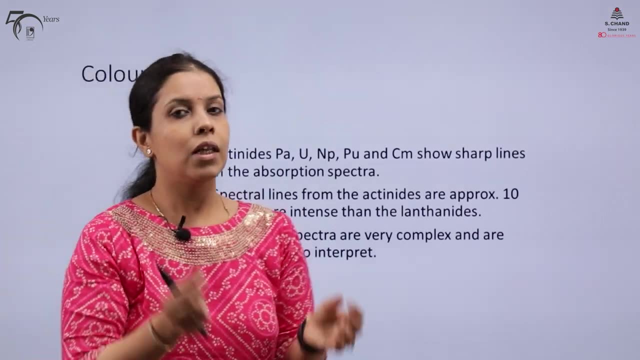 due to transitions. color will show which color will show whatever color is being absorbed by that particular element, then its complementary color. we will be able to see that the color, the absorption, should be in the visible region so that we can see that. 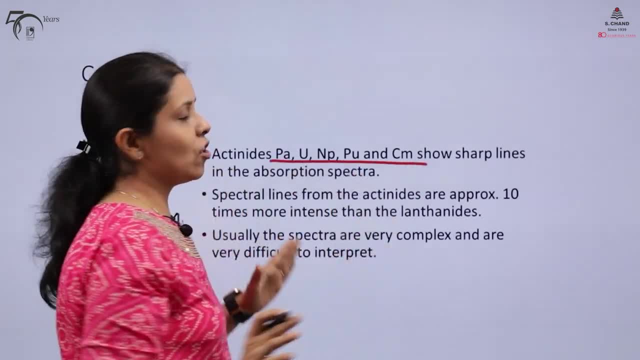 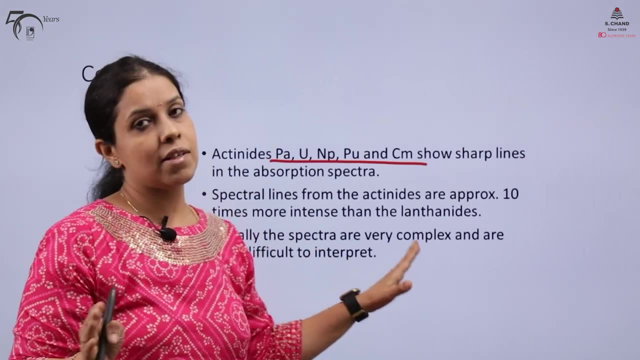 so there are some compounds, actinides, which show us sharp lines in absorption spectra. spectral lines from the actinides are approximately 10 times more intense than the lanthanides. ok, so the lines of actinides are very sharp. 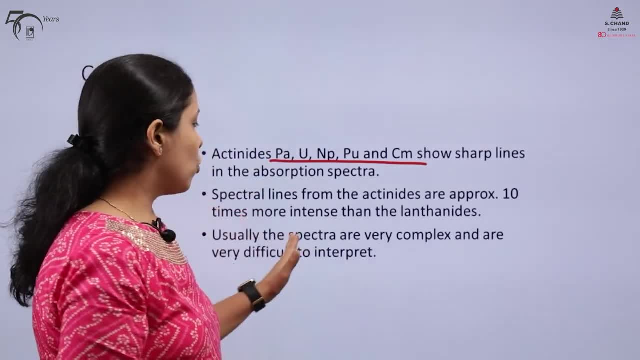 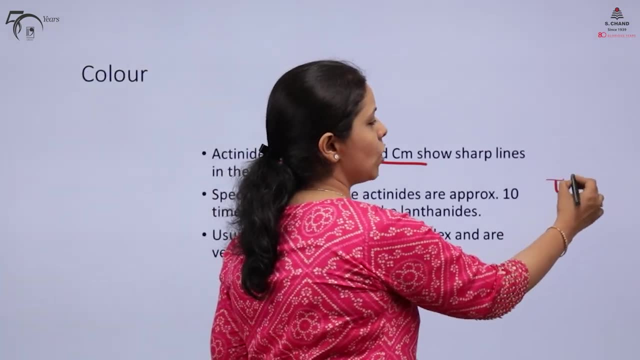 but usually the spectra are very complex. so because there can be a lot of transitions in this F orbital, a lot of oxidation states are showing. in the case of lanthanides, usually plus 2 and plus 3 oxidation states were there. 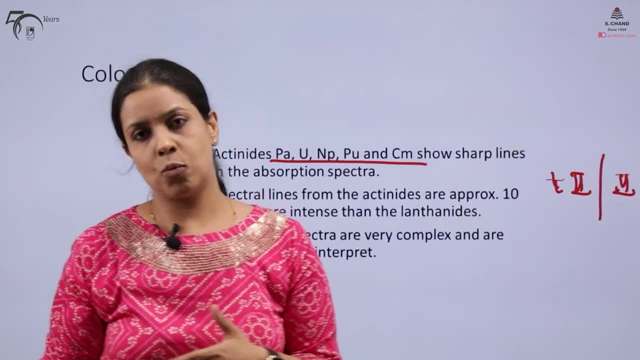 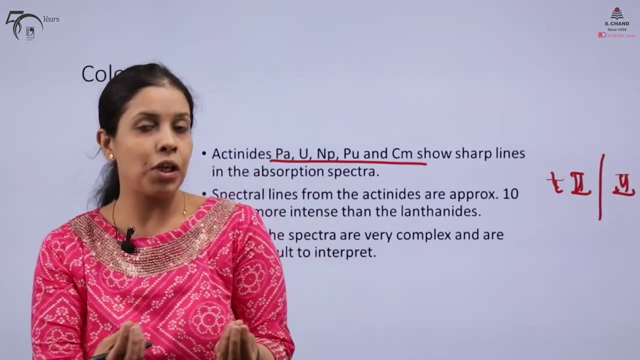 right, but in this case a lot of oxidation states are possible, so a lot of transitions are happening. so the spectra are very complex. it is very difficult to interpret them. from where, from where which low energy goes to the high energy orbital? 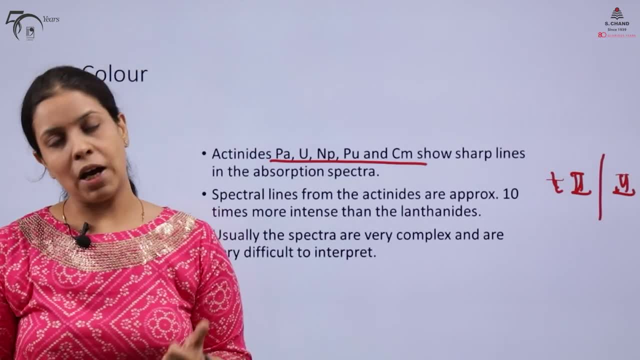 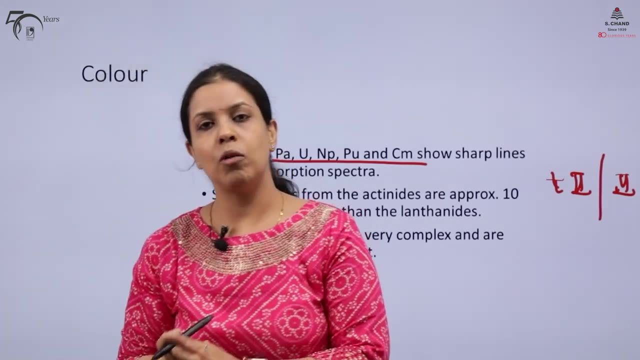 it is very difficult to interpret otherwise. they show colors and their magnetic properties also show, as we have already discussed, and in this case also we have. we consider the orbital motion and the orbital motion and sometimes the spin-orbit, coupling happens. 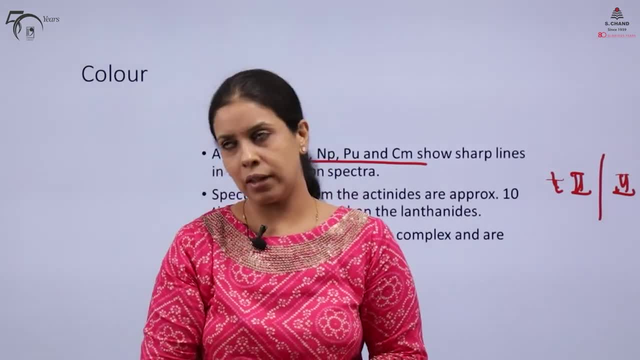 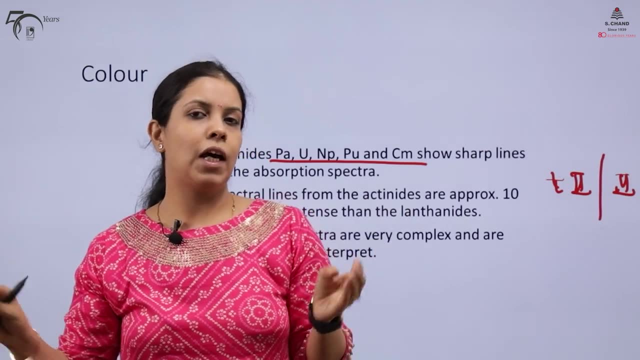 so, on the basis of the new quantum number J, we also get the magnetic moment. just like there is a lanthanide contraction, the same way there is an actinide contraction. we get to observe the study decrease and after that. 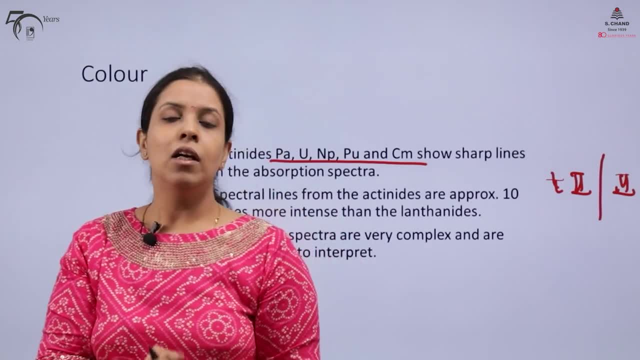 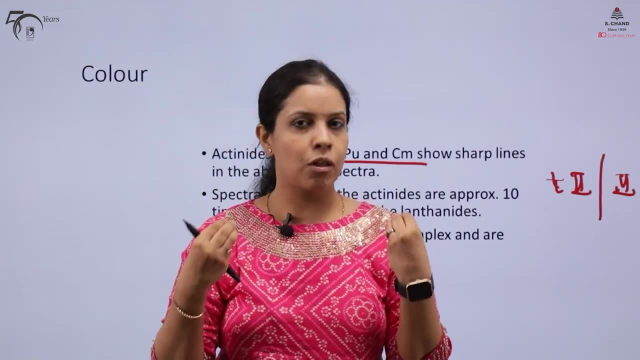 we get its effect in the transition element series right. so in this video we have discussed all about lanthanides and actinides, so I hope it is clear to you how they are showing different oxidation states, how they have electronic configuration. 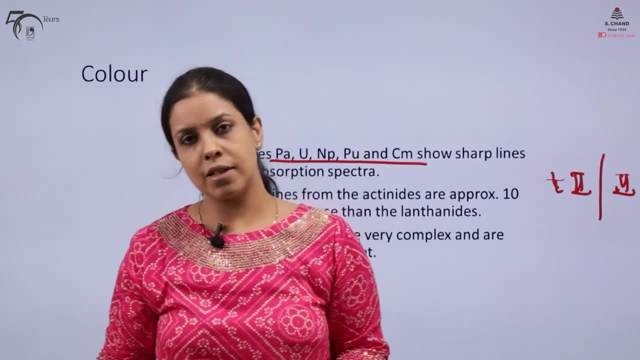 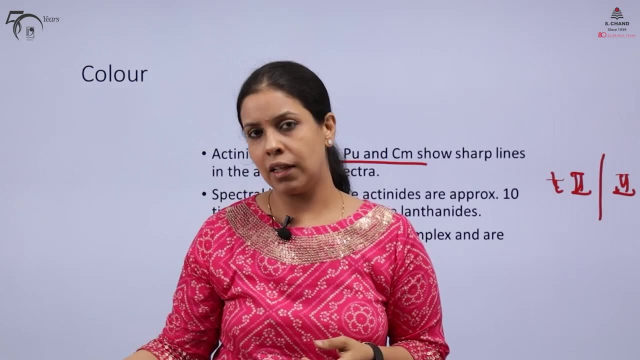 why they show colors, how you can separate lanthanides. we have discussed the ion exchange method, which is a very important method for you to understand. then we have discussed lanthanides contraction. lanthanides contraction has a very similar actinide contraction.